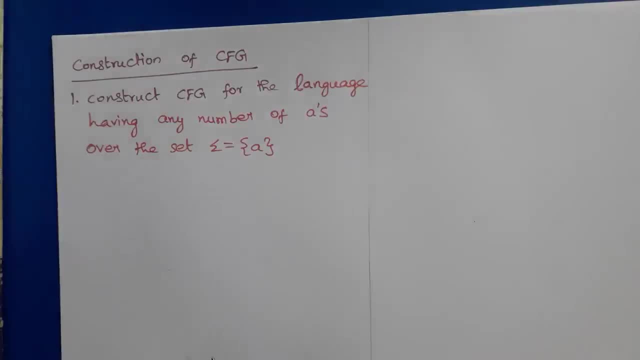 Hello all. in this lecture we are going to discuss about construction of CFG for some example problems. So the first one is construct CFG for the language having any number of a's over the set sigma is equal to a Sigma. the input alphabet has a single input symbol. 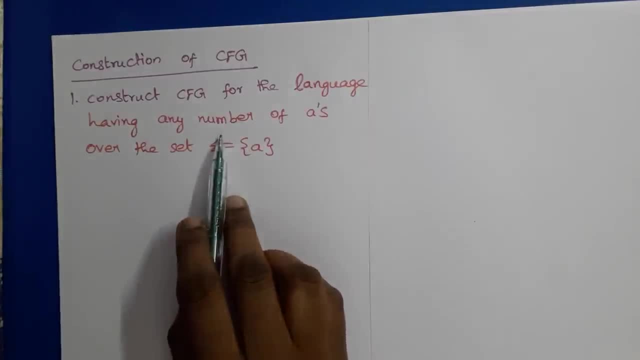 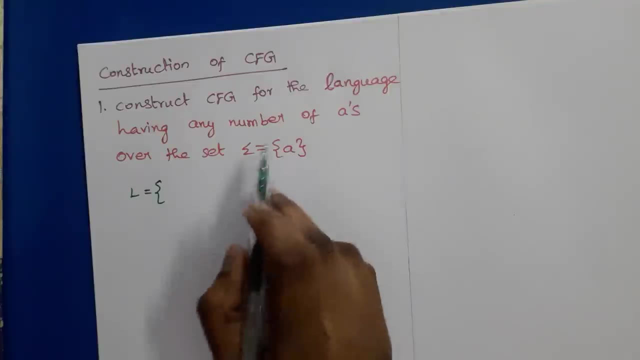 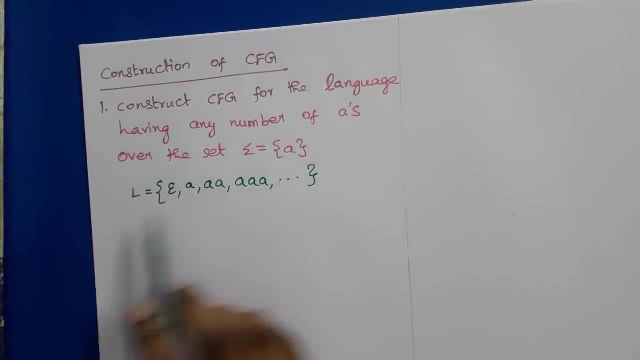 a and the language should accept all strings which consist of any number of a's. So what is the language of this grammar? Any number of a's, so including epsilon, So 0 number of a, 1 a, 2 a's, 3 a's, etc. So our CFG should accept all these strings: epsilon single a. 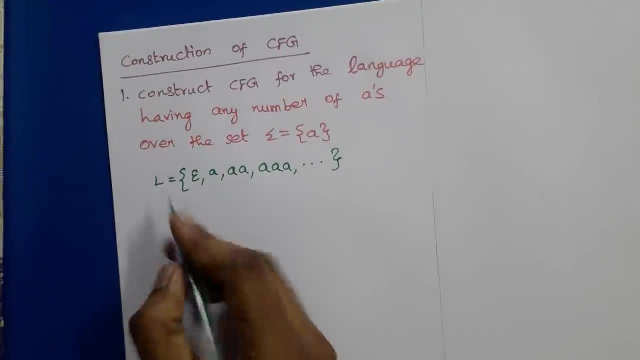 double a's, 3 a's, 4 a's, etc. So how to construct context, free grammar for this: Yes, starting symbol of the grammar. For example, we are going to consider yes, Yes tends to, yes tends to a, and we need to. 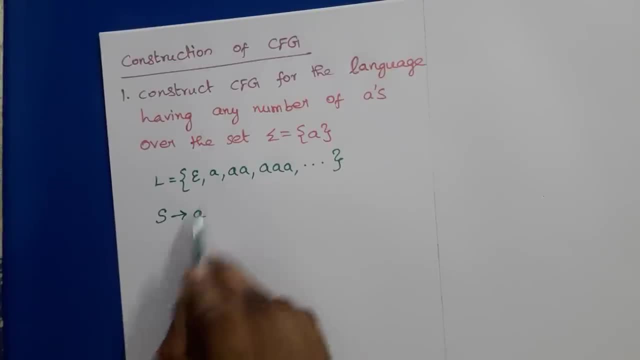 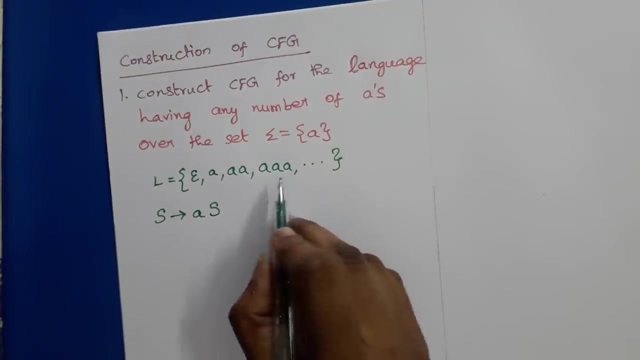 get repeated a's right, any number of a's, So a should be followed by yes, right. This is for recursive step, So any number of times we can replace yes by a yes, a yes, a yes like that. So if we try to derive 4 a's means, how can we draw the parse tree? We will start. 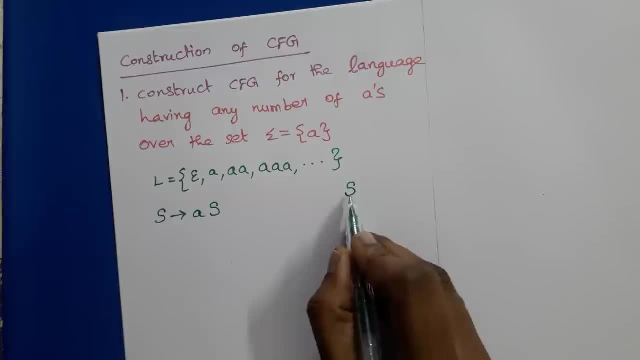 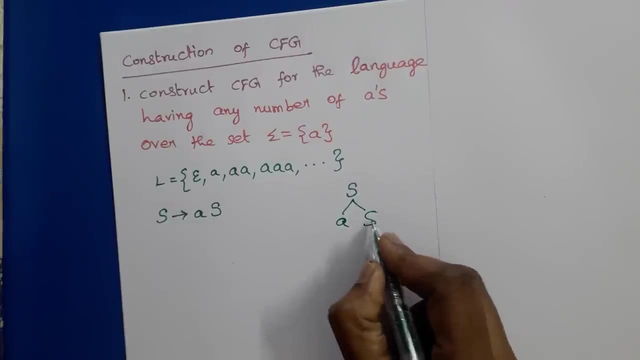 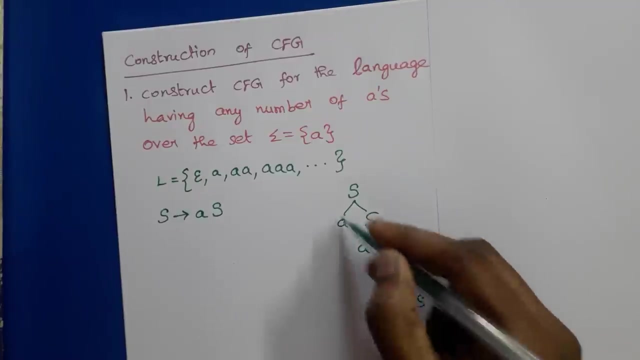 with the starting symbol of the grammar a and yes. sorry, start symbol of the grammar yes, and this yes can be replaced by a yes, the production a yes. and again this yes should be replaced by a yes, a yes, a yes. So we have got 4 a's, but finally it should be stopped. 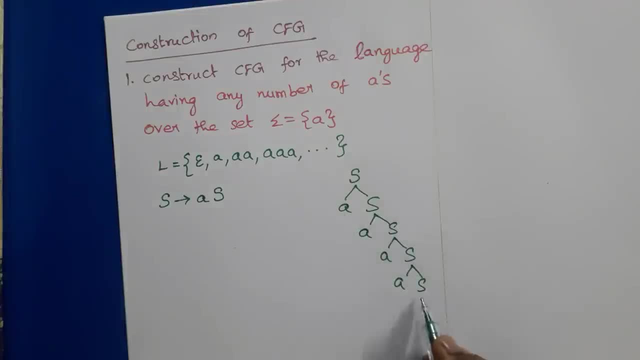 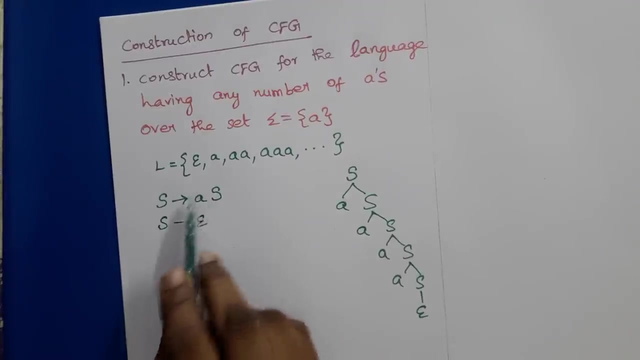 right, because the string should consist of only the terminal symbols. So it includes epsilon also, right? This language includes epsilon also, So that it should be finally replaced by epsilon. So another production is: yes tends to epsilon. Okay, so yes tends to a. yes, Any number of a's means we have to write yes, start. 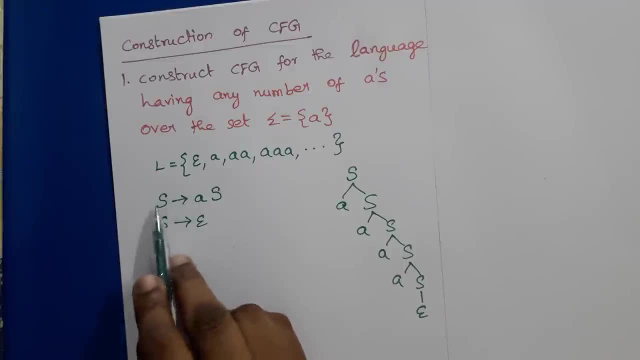 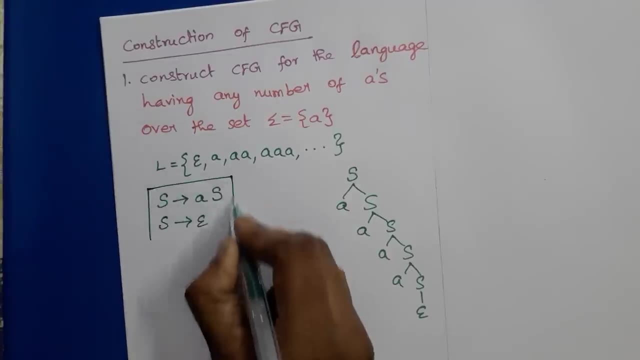 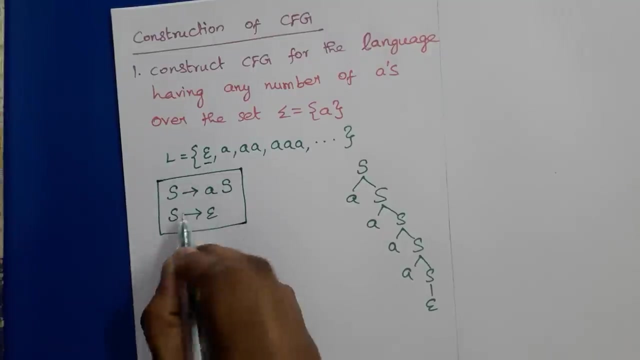 symbol of the grammar: tends to a variable, tends to a and the same variable. This is the recursive step and this is the basic one. So, yes, tends to epsilon. So this is the. these are the two productions for getting this grammar. So if we want to derive this string, then we 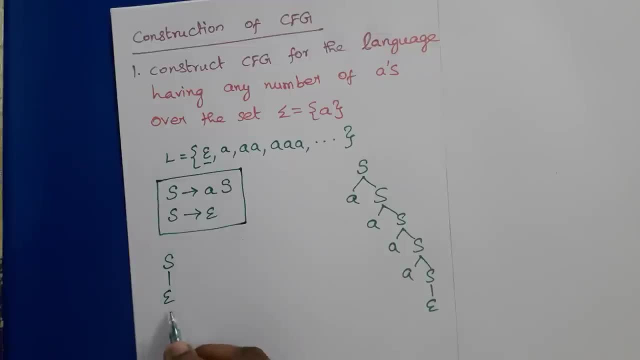 will get. the starting symbol of the grammar should be replaced by epsilon directly, So we can get epsilon. If we want to get single a, then yes must be replaced by a yes. once, Once we have to use this production, then this yes must be replaced by epsilon. So if you 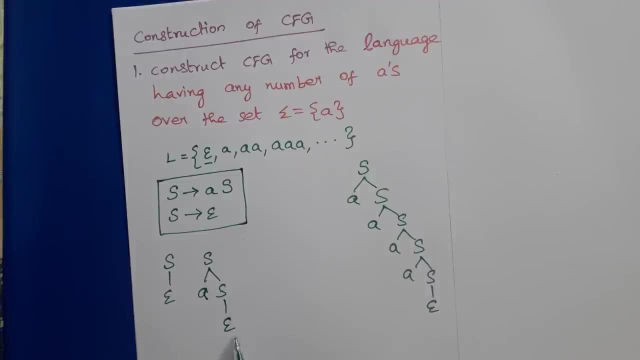 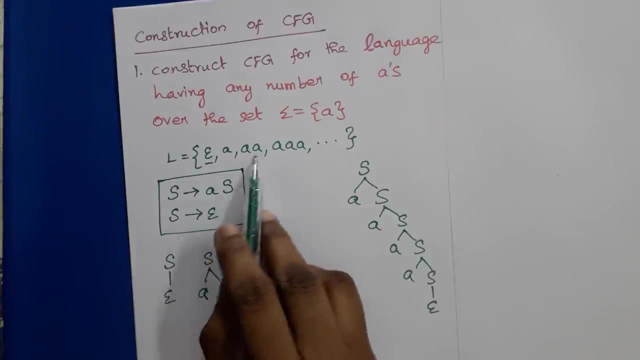 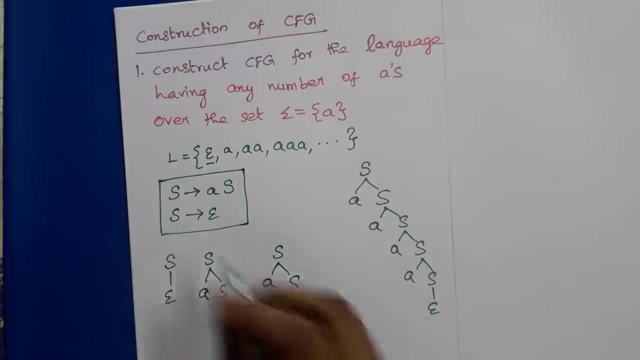 concatenate this, we will get single a. Okay, epsilon is an identity element during concatenation, So if we concatenate the leaves, we will get single a. Similarly, double a. This string means yes must be replaced by a yes. Again, this yes must be replaced by a yes. We need 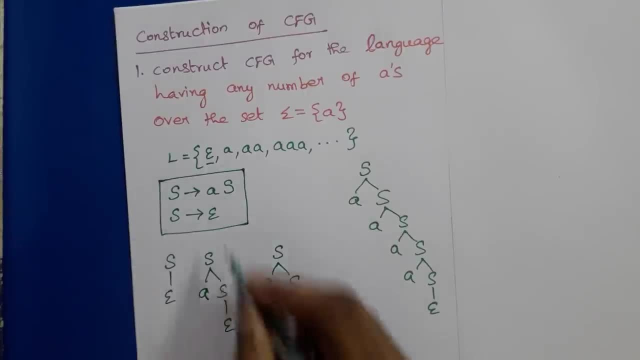 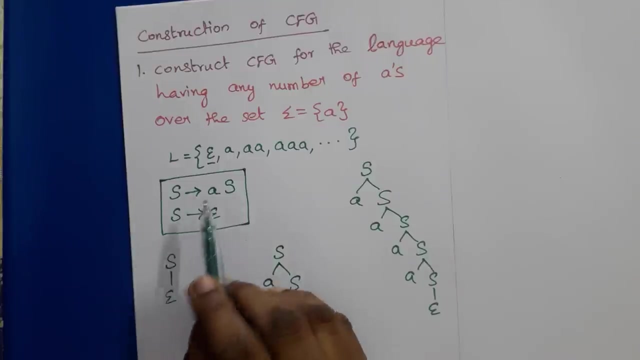 to use this production as many times as we want. Finally, it should as many a's we want. Then, finally, yes, must be replaced by epsilon. So double a. Similarly, for three a's means three times we have to use this. Then, finally, it should be replaced by epsilon. So the grammar. 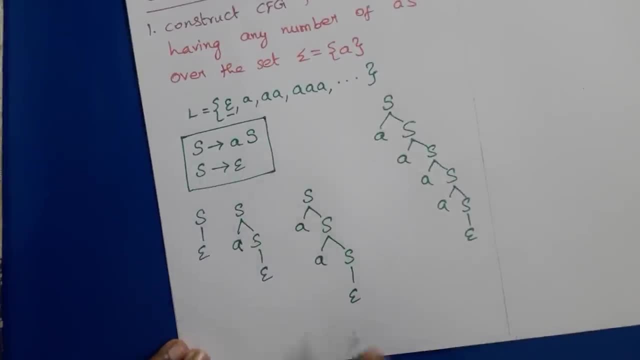 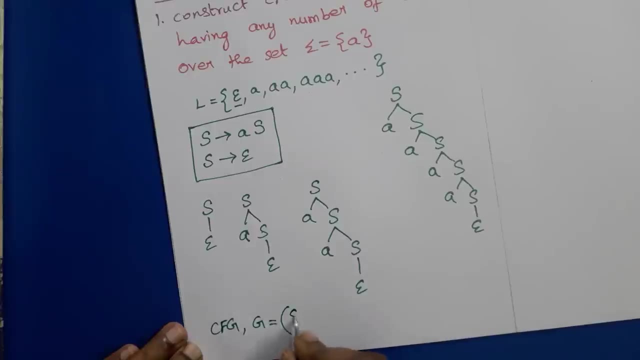 the set of productions. for this grammar is yes, tends to a yes, and yes tends to epsilon. Okay, But how to write the context? free grammar notation as a five tupule. So CFG G is equal to VTPS, V is yes. here Terminals are a alone. It is given in the question. Then set of productions. 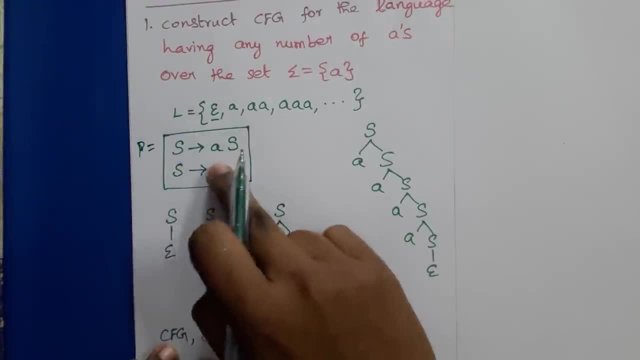 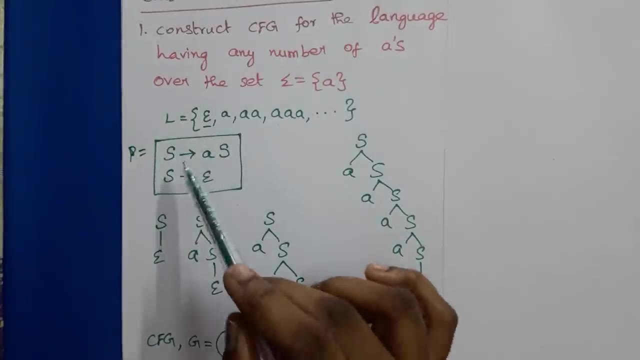 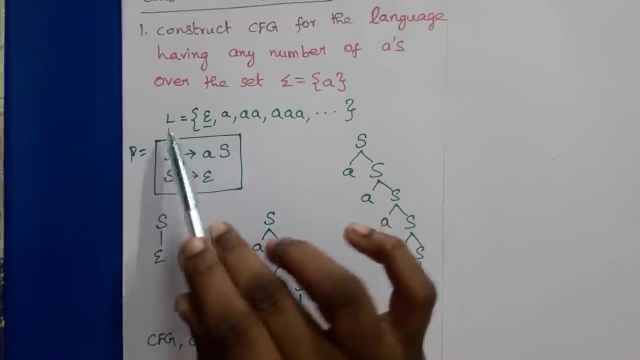 P that we have written. So these are the set of productions. Then start symbol of the grammar is also yes. So construct CFG means we have to write this four tupule notation. So we have a four tupule notation and set of productions. This is for your understanding. We can write: 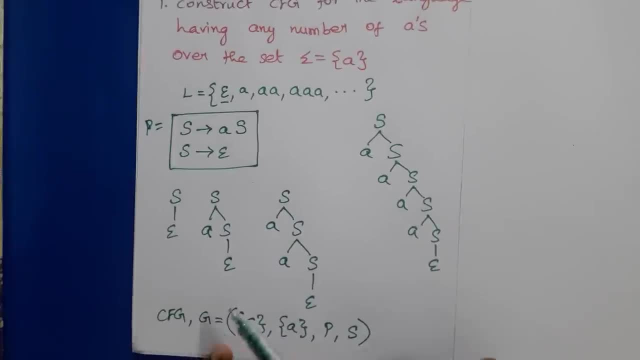 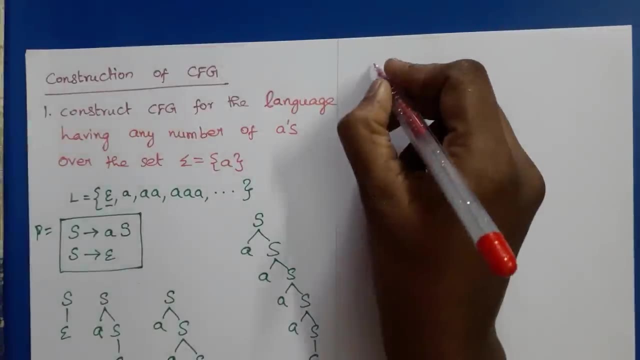 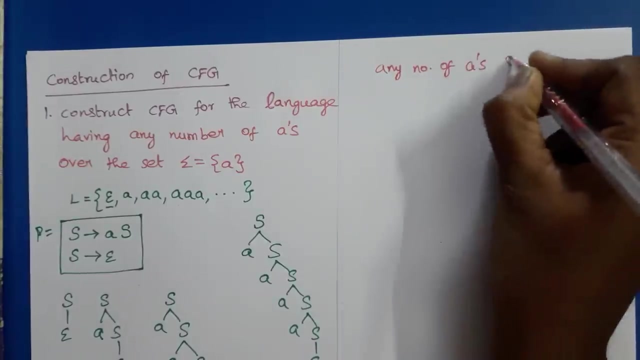 language and try to derive the productions 1st, Then we can write the four tupule notation. Then next we will see another example. Suppose if we want to construct a language for any number of A's and B's. any number of A's and B's means what is the language? the last five: 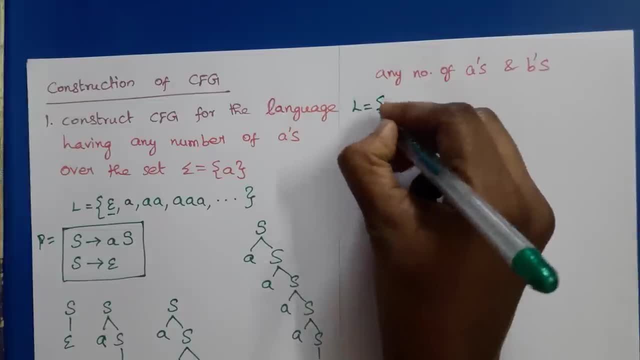 ones, So you can imitate it. So it is played that So, if, say you have this Ganze of B's what the last five numbers are, say, so that means this is a total number of As, if that Yas, and this means both As and B months в. Well, the free Q знать that needs to change from the 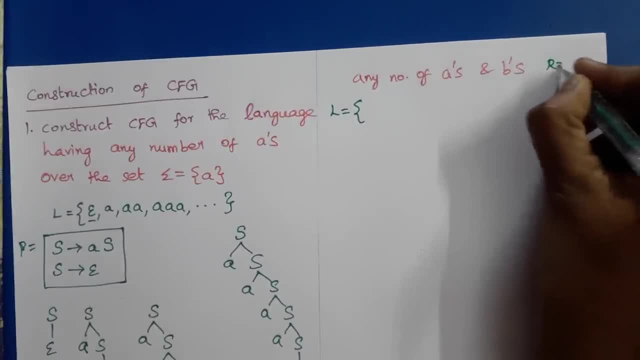 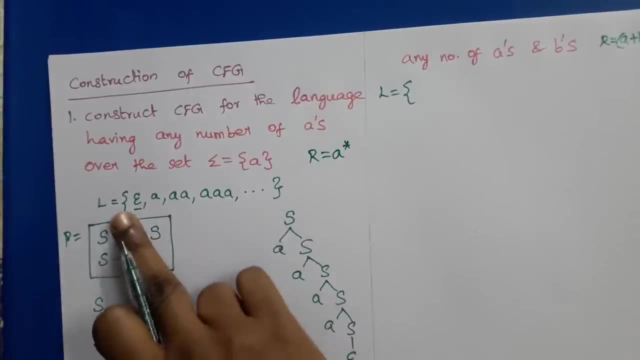 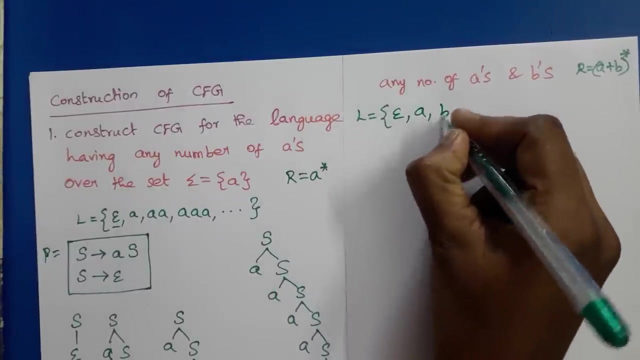 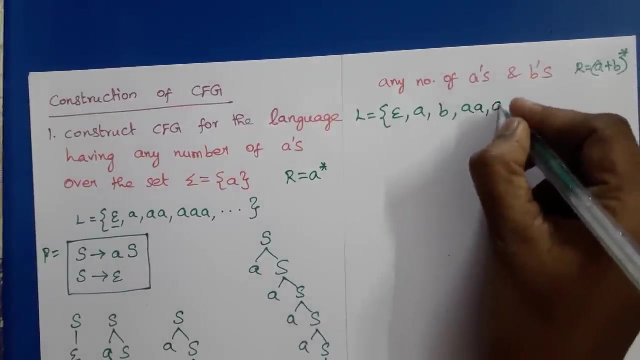 the meaning is: regular expression: is a or b star. right here, what is the corresponding regular expression: is a star. so we have got this language and any number of a's and b's means epsilon a, b, epsilon a, b and any combinations of a's and b's, right. so a, a, a, b, b, a b, b. this is the zero length. 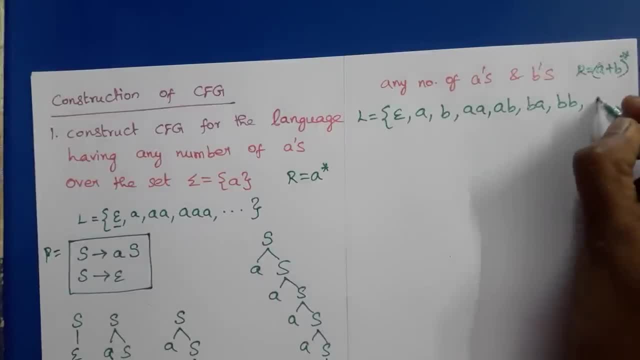 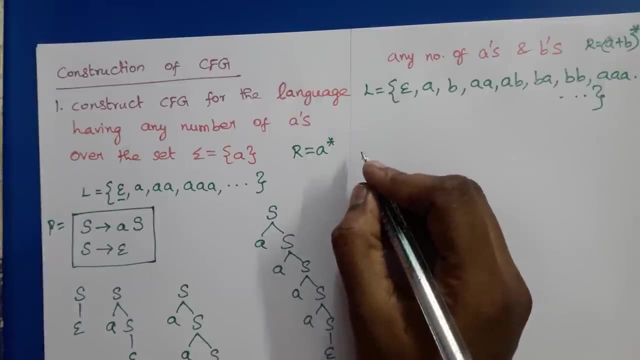 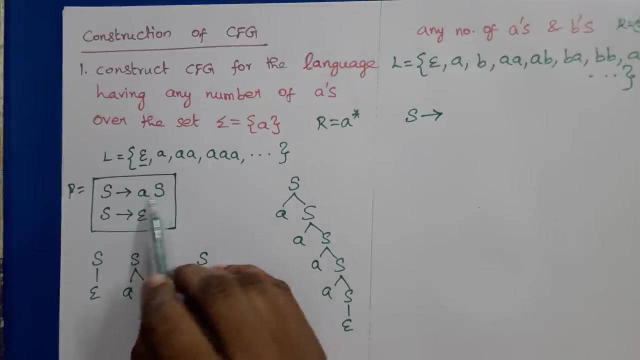 string. one length strings, uh, two length strings, similarly three length strings, and so on. so any combination of a's and b's. so now we need to write the set of productions for this grammar. so yes, tends to any number of a's means we have written like this, right. so a s bar any number. 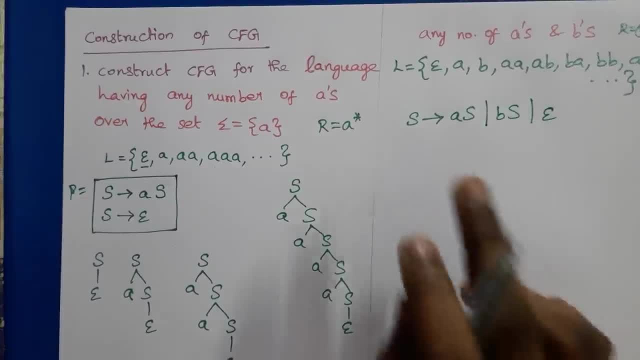 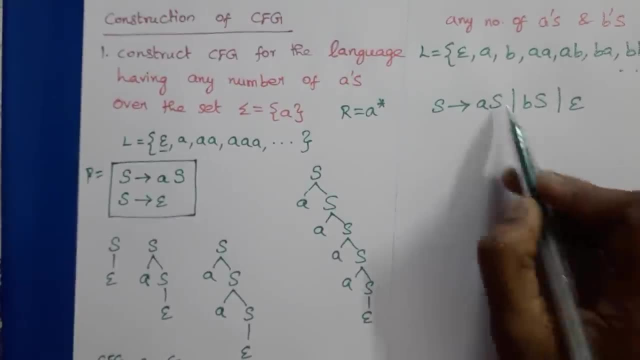 of b's means b s bar epsilon. and one more thing: if the two productions are having the same heading, then we have to write the set of productions for this grammar. so a s bar epsilon means we can combine by using this vertical bar, so this production can also be written as: 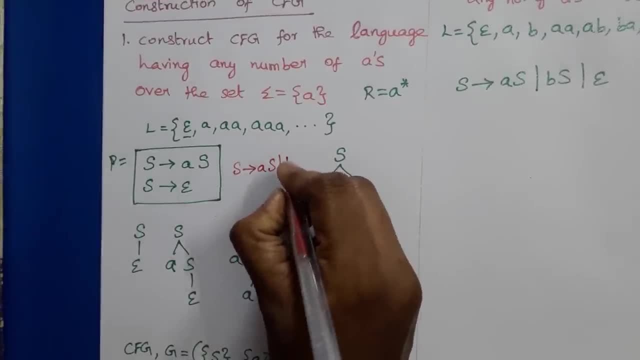 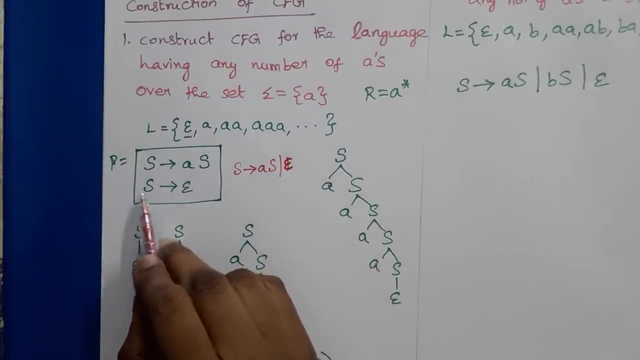 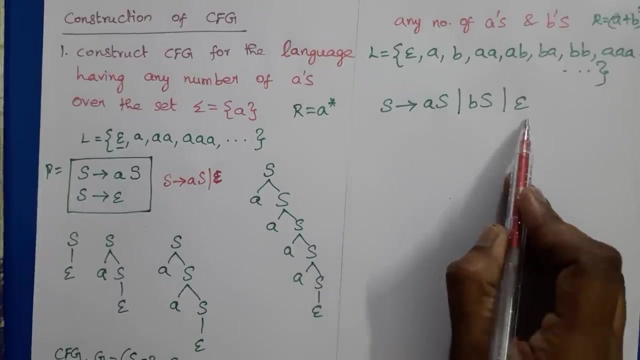 s tends to a s bar epsilon. sorry, because these two body um are having the same left side head. so s tends to a s bar epsilon. so s tends to a s bar b s bar epsilon. so if we want to get a, b a b, then suppose a, b a b. if you want to get a, b a b, then suppose a, b a b if you want. 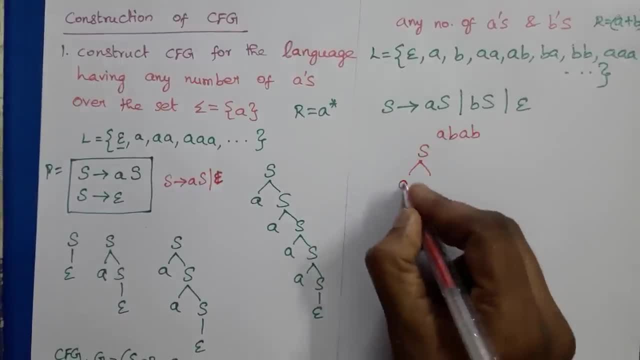 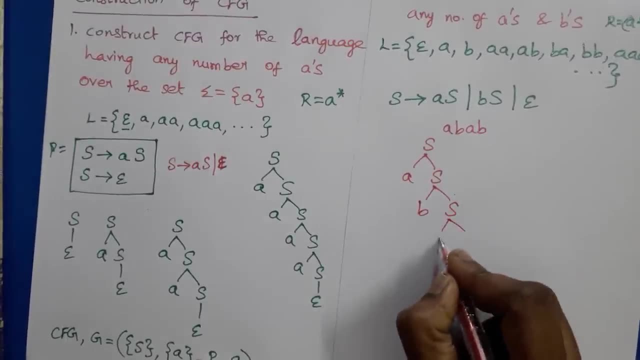 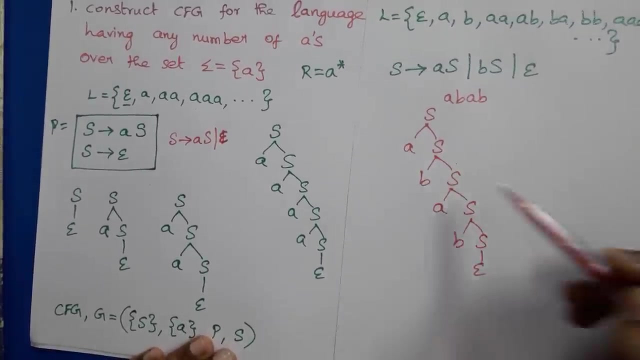 to get it. then yes tends to yes, can be replaced by a s. first this s must be replaced by b s, then this yes must be replaced by a s, then again b s, then finally epsilon. so we have, we got a, b, a, b. so any number of a's and b's means this is the um grammar. okay so, but i i am going to write the. 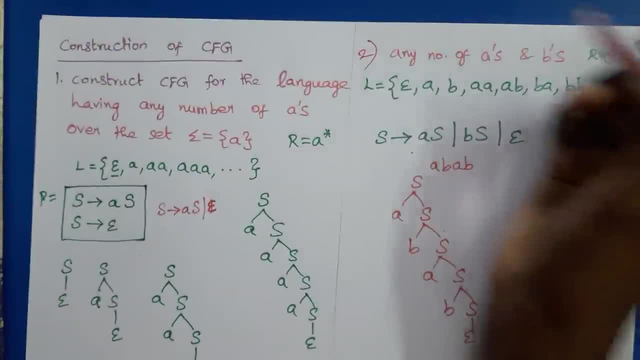 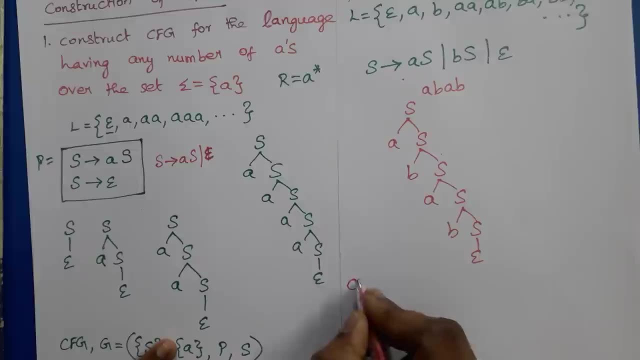 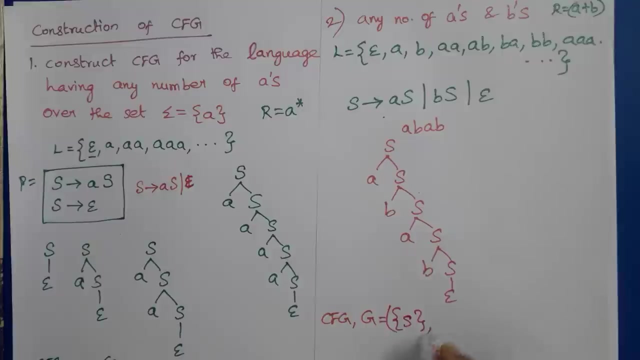 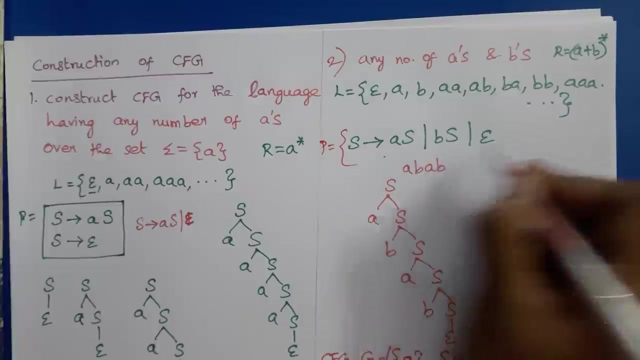 productions for all the examples. but you need to write the four-tipule notation of the four-tipule notation also. okay, i'll write it here. so cfg g is equal to variable terminals a and b. set of productions p. this is the set of productions. then start. 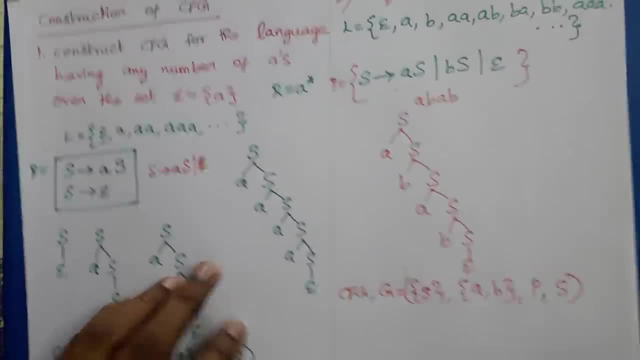 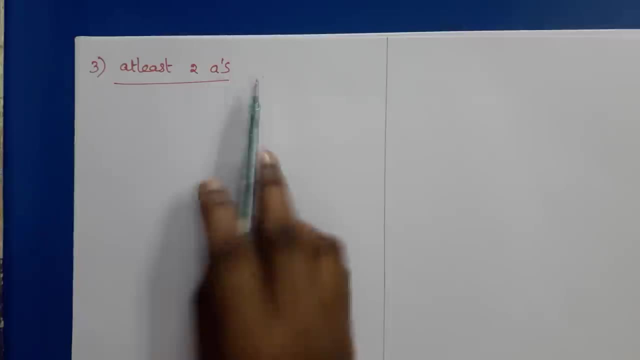 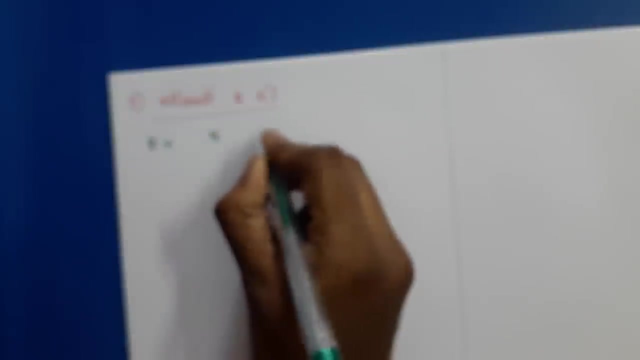 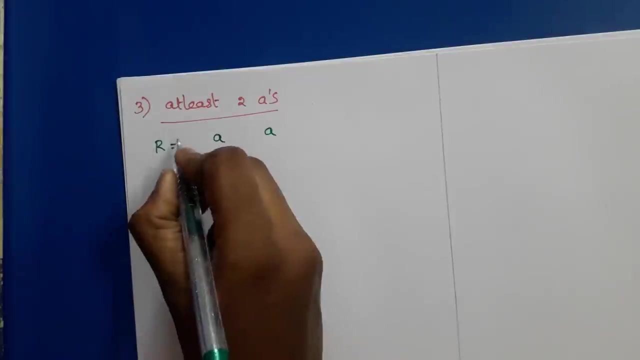 symbol of the grammar is yes, then write the productions. next one: construct a cfg for the language contained in the grammar strings of at least two a's. so how to construct a regular expression for this. at least two a's means two a's are compulsory in each string. two a's are compulsory, right. this a can be preceded. 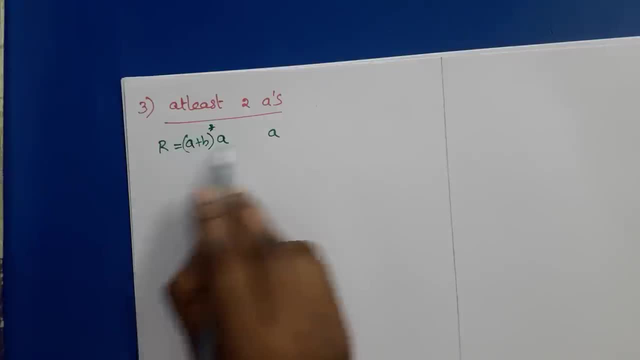 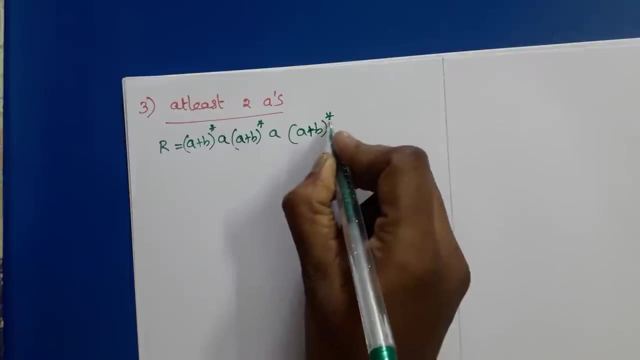 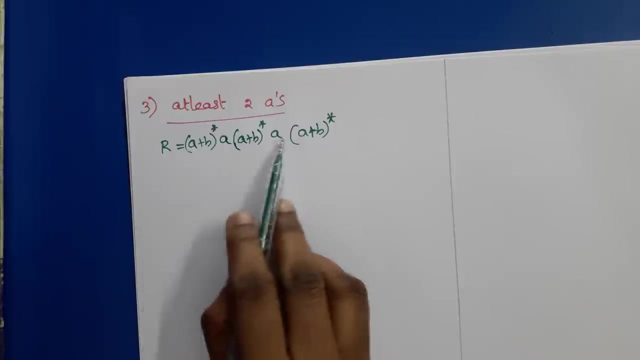 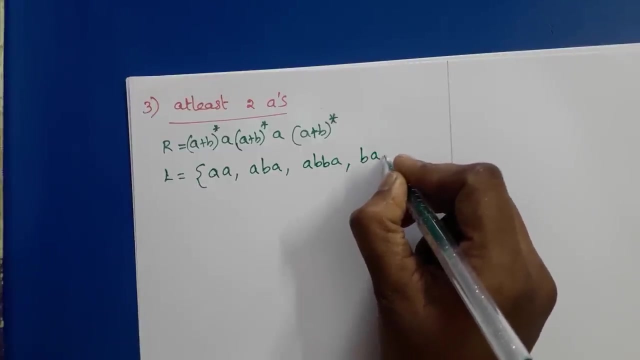 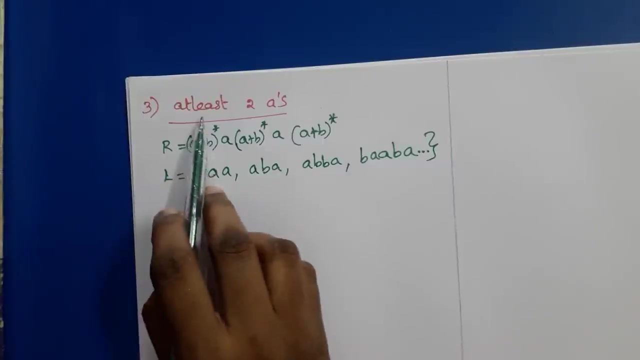 and followed by any number of a's and b's. right, these two a's must be preceded and followed by any number of a's and b's. so this is the corresponding regular expression for this problem. Now we need to construct the CFG right. all the strings should contain at least two a's, so it can be preceded and followed by any number of a's and b's. so, for example, a, a is a correct input string. a, b, a, a, b, b, a, b, a, a, b, a. okay, so these type of strings: the string has three a's, but the condition is at least two a's. 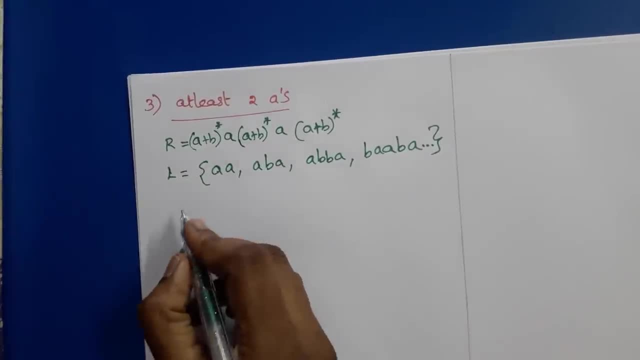 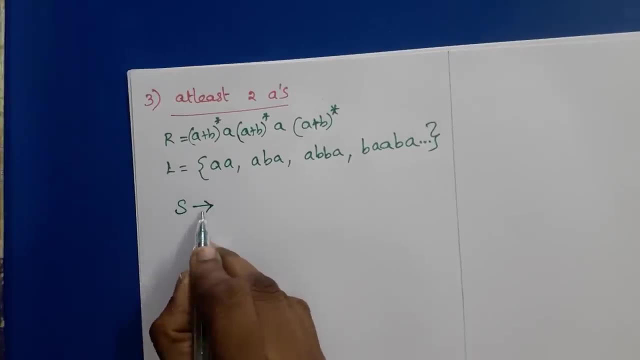 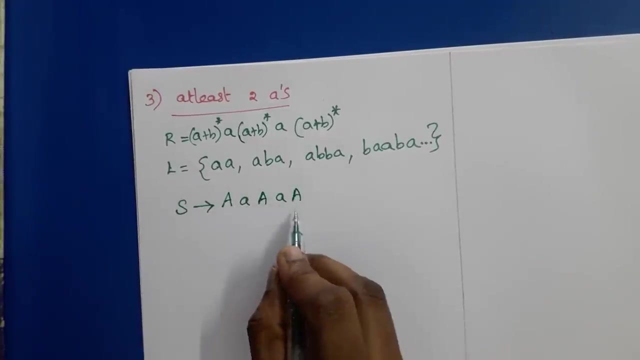 So all these strings are correct input string. so now we will try to construct the CFG. so assume that yes is a start symbol of the grammar. so, yes, two a's, right, two a's are compulsory. it should be preceded and followed by a plus b star, right? so for that we are going to introduce another variable, capital a. okay, so two a's are compulsory. this a should be written as: 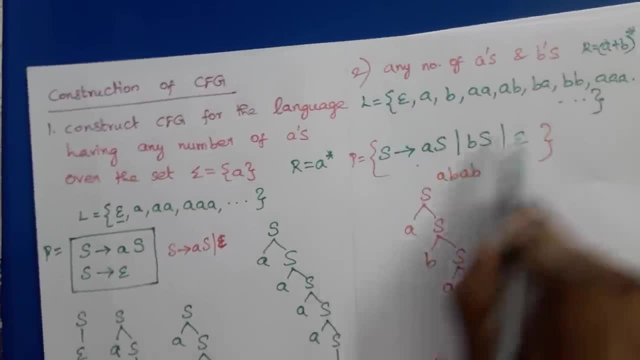 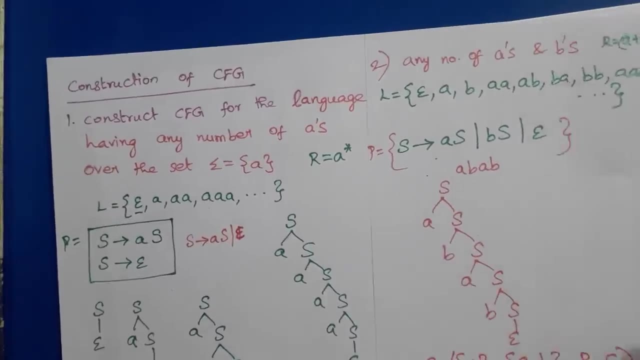 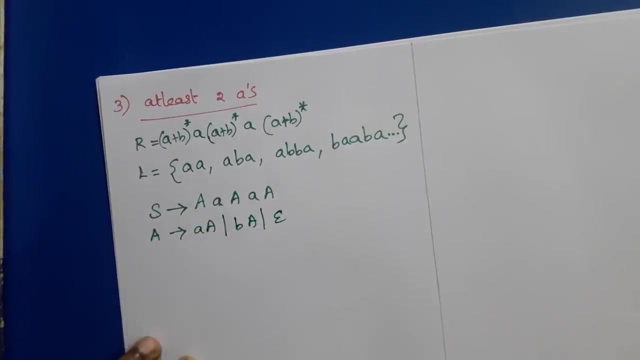 a plus b star, any number of a's and b's. any number of a's and b's means what is the? this is the production right. yes, tends to a s, bar, b s, bar, epsilon. here the variable is a, so a, a, bar, b, a bar, epsilon. so this is the set of productions for this particular grammar right, at least two a's, and it can be preceded and followed by any number of a's and b's. 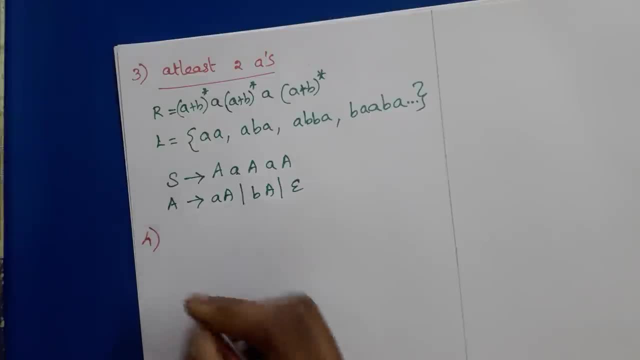 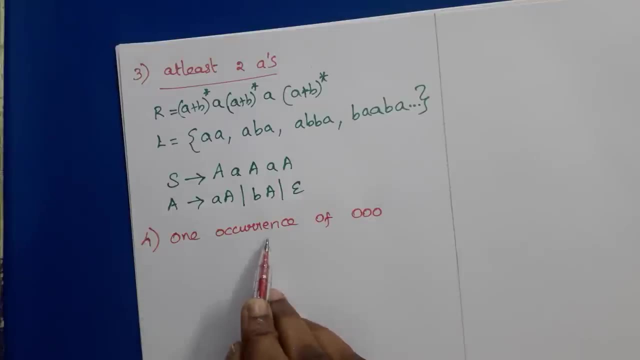 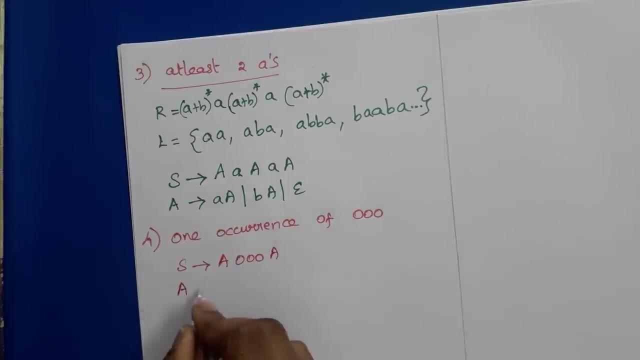 Then the fourth problem is One occurrence of triple zero. all strings, the language in which all strings are having one occurrence of triple zero. so how to construct CFG for this? yes, tends to triple zero. this is a substring we need to get in the string. it can be preceded and followed by any number of zeros and ones, right. so for any number of zeros and ones, we need to introduce a non terminal a and this is a sub string. 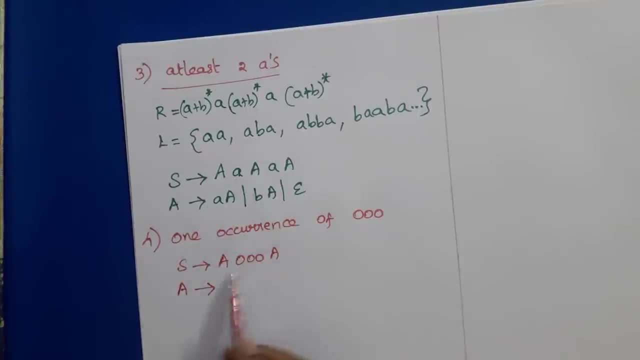 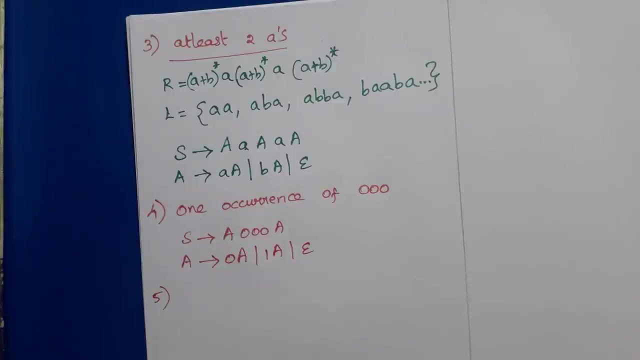 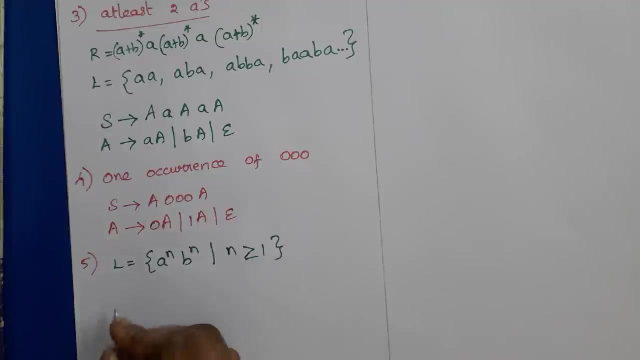 And this is a, can be expanded like this. any number of zeros and ones here, a's and b's, zeroes and ones, so zero a, any number of zeros can be retrieved from this, any number of ones, and epsilon. okay, then the fifth problem. L is equal to a to the power n, b to the power n, such that n is greater than or equal to one. so the set of strings are a, b. 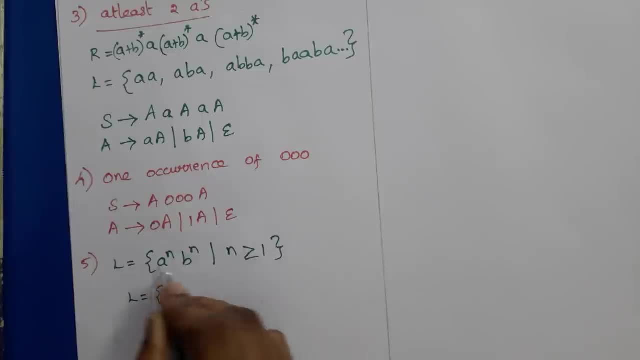 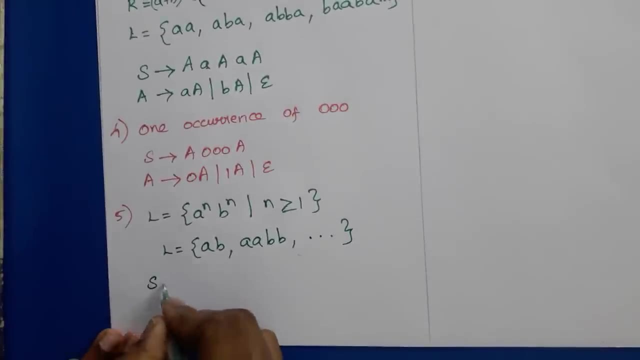 Because n is greater than or equal to 1, so a b if n is 2, double a, double b, etc. so how to construct a cfg for this? yes, tends to. number of a's must be followed by number of b's, and it's the numbers should be. 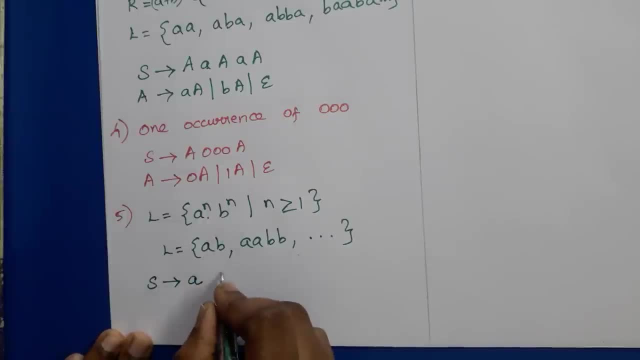 equal right. so for 1 a we need to get 1 b right and it should be recursively retrieved, so small letter a s b. so a s b, a s b repeatedly can be applied. okay, suppose, if i want to get the string from this grammar. so yes, can be replaced by a s b, then a s b. so a a b b. but i have 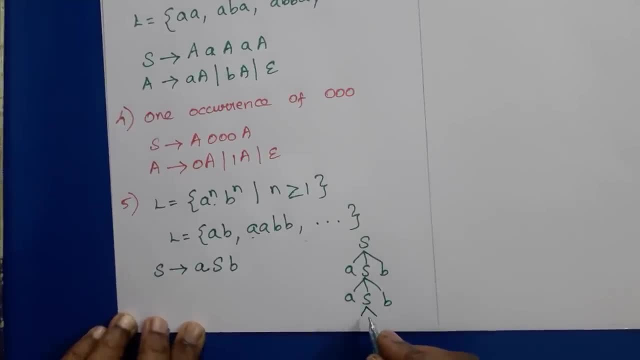 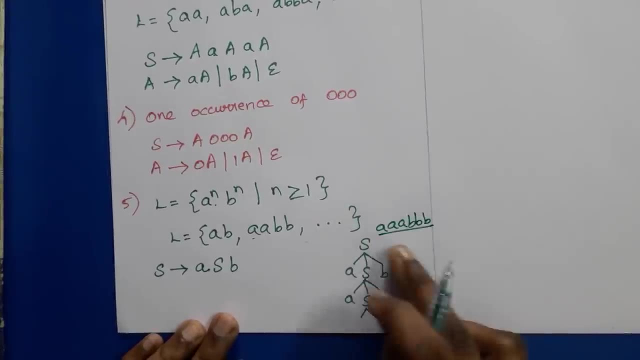 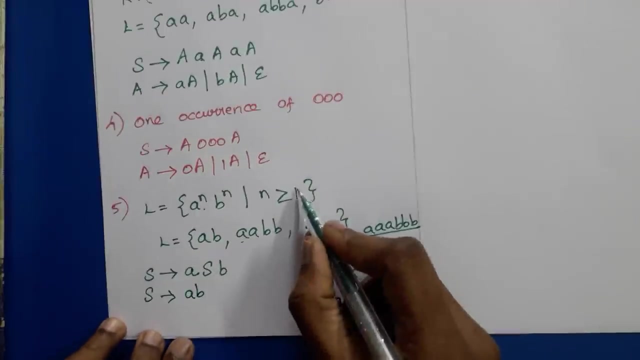 to stop this right. so it should be replaced by. it cannot be replaced by epsilon, actually. okay. so this is the parsery for getting 3 a's, 3 b's. okay. so a b, yes, tends to a, b should be replaced. suppose here 0 is given, then we can write s tends to epsilon. so how to get double a, double b. 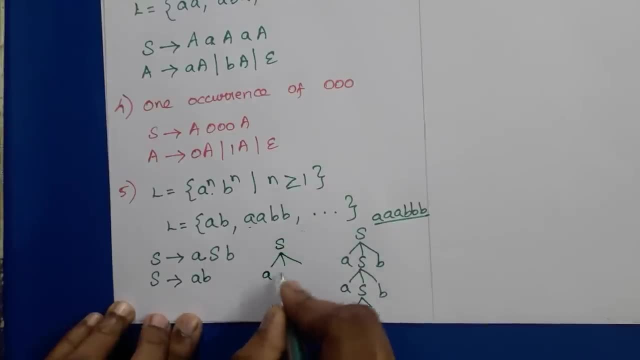 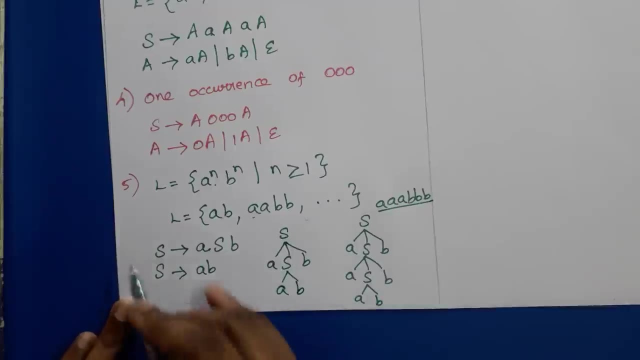 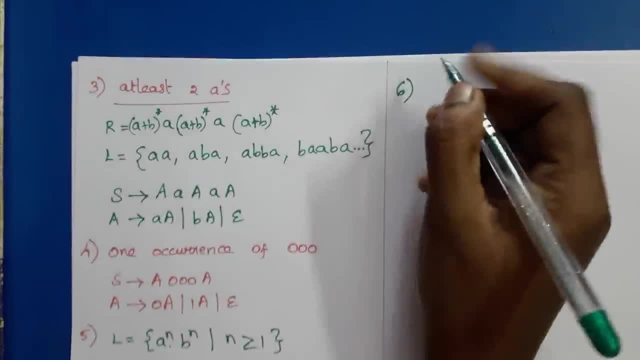 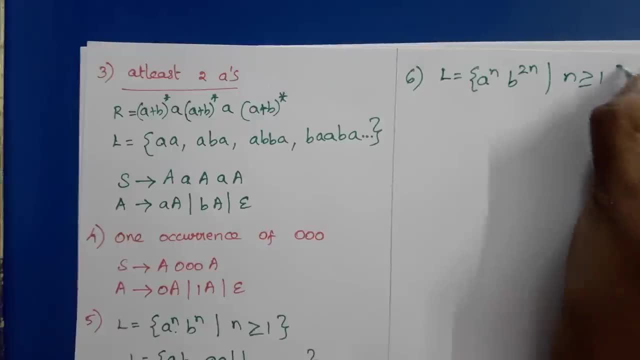 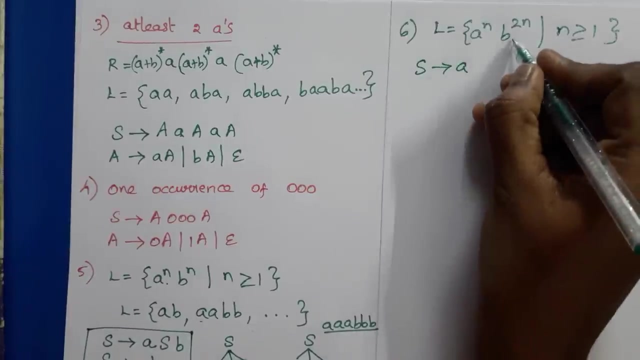 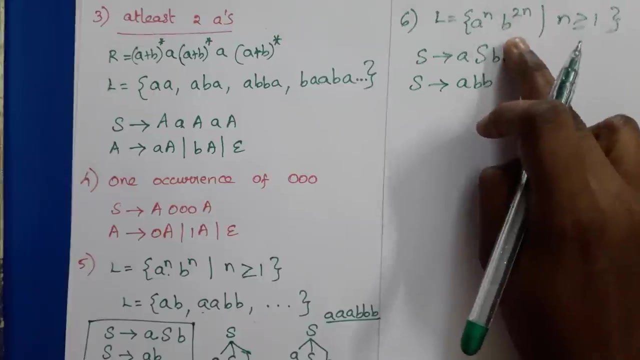 n. suppose if we want to construct cfg for a to the power n, b to the power, 2 n, then that grammar is similar to this. but for 1 a we need to get 2 b's right, so a s, b, b, then s tends to a, b, b. similarly we can construct cfg for this type of problems. the next one: 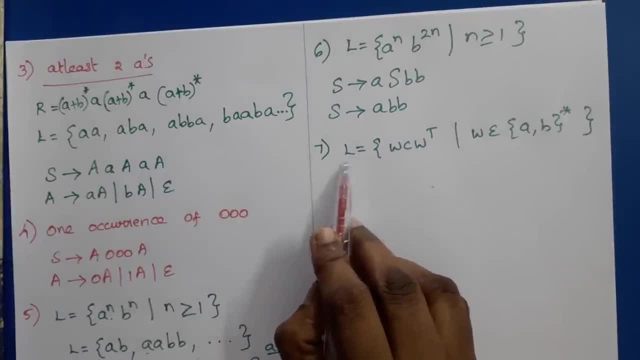 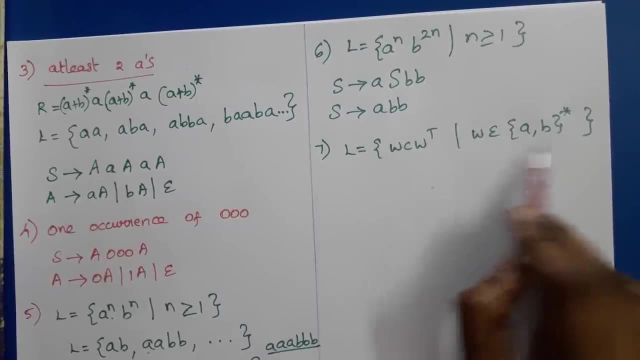 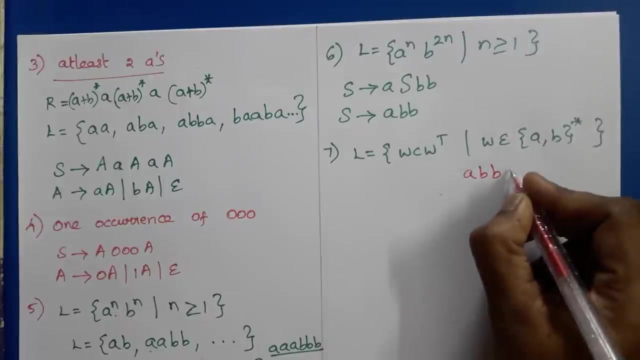 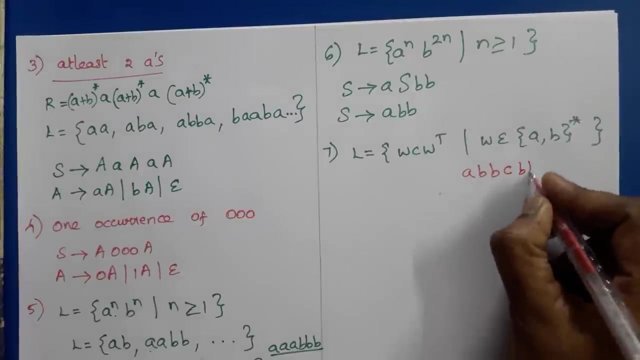 another problem is construct cfg for this language. l is equal to w, c. w transpose in such that w belongs to a comma, b, star, any number of a's and b's. so if we have got a, b, b as w, then it should be followed by the center c. then w transpose: this is w, so transposes b, b, e, right, so this is a palindrome. 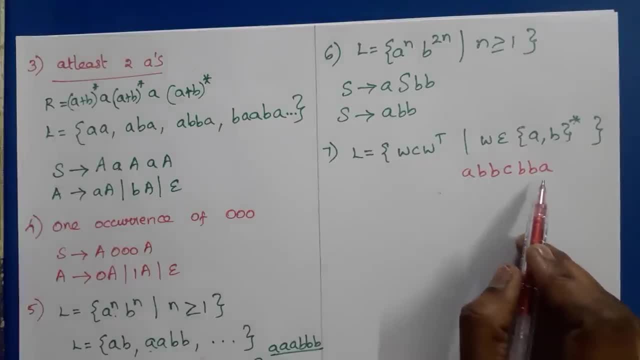 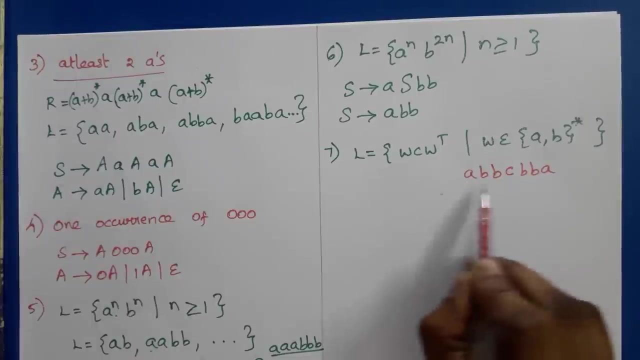 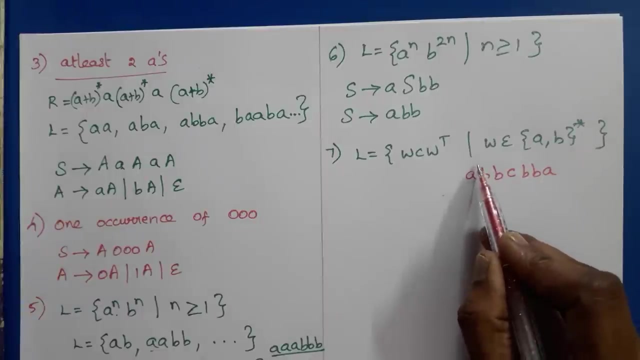 string. actually this one is an odd length palindrome with the center marker c. so here palindrome means we know that the string. if we read the string forward and backward it will give the same answer. and one more thing: the string, palindrome, string starting and ending with the same symbol. and if you remove the 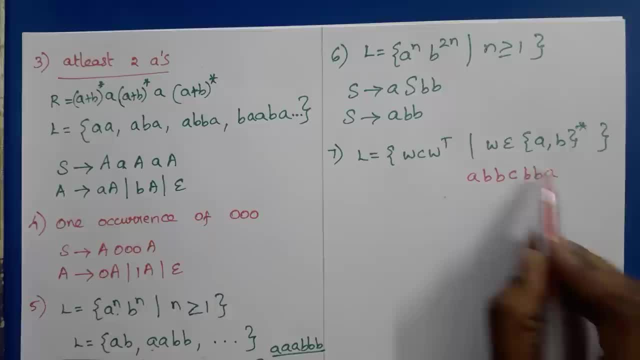 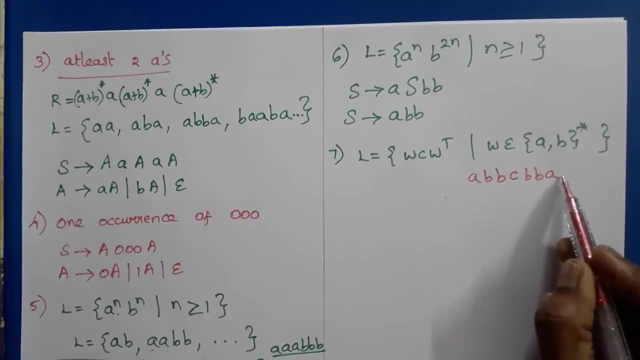 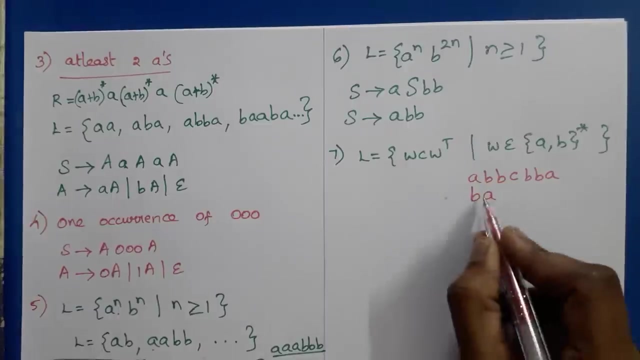 start symbol and ending symbol in the remaining string. also, starting and ending symbol are same right. so if the string starts with a, it should end with a. if the string starts with b, it should end with b. right suppose if another example b a, in which the w is b? a and the center marker is c means what? 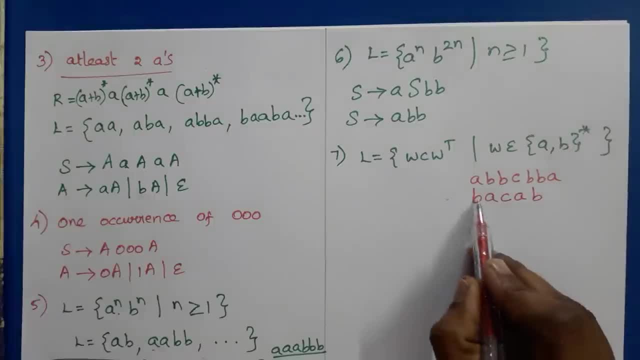 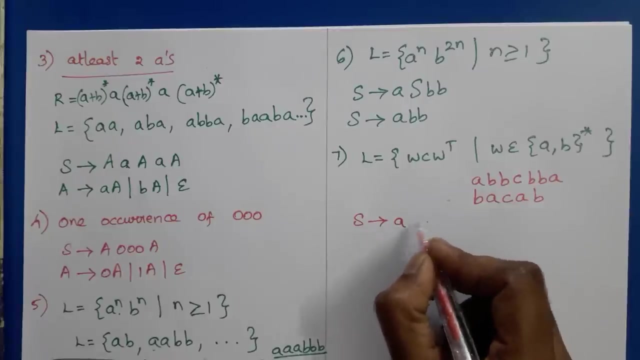 about w, reverse a, b, right. so if it starts with a, ends with a, starts with b means ends with b. so how to construct context-free grammar set of productions? s tends to a. starting with a means ending with a, for recursively we need to retrieve this. so a, yes a. if it starts with b, it should end with b. 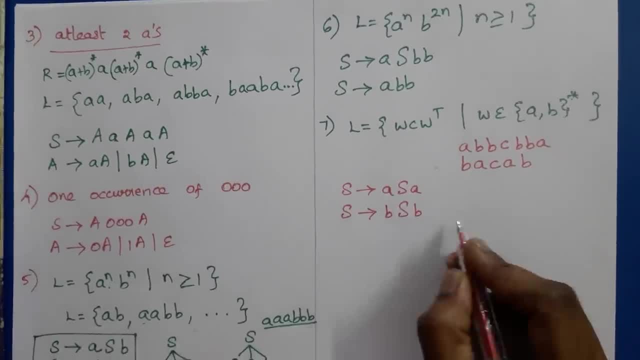 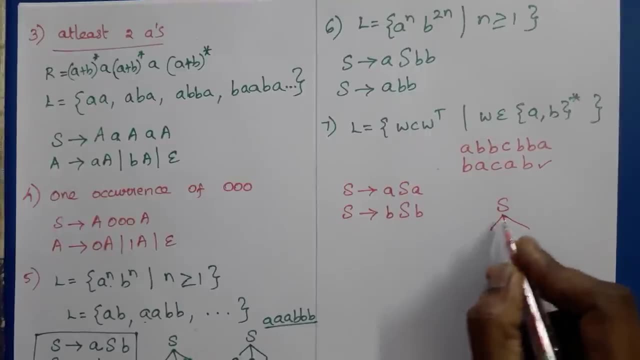 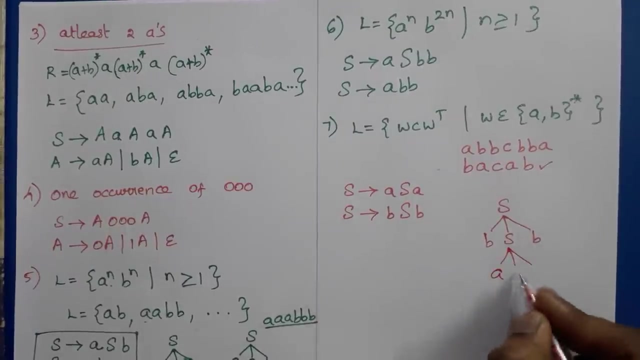 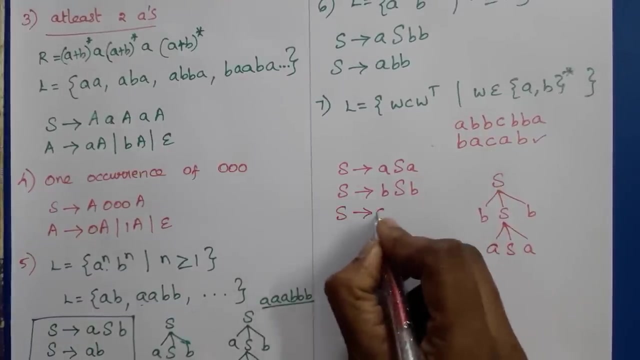 so if we try to construct partially for this, this string yes must be replaced by b s, b. then we need a, so yes must be replaced by a, yes, a. finally, it has to be stopped right. so the center symbol is c, so yes tends to c must be the production. then only we can get b a, c, a, b. similarly we can draw for: 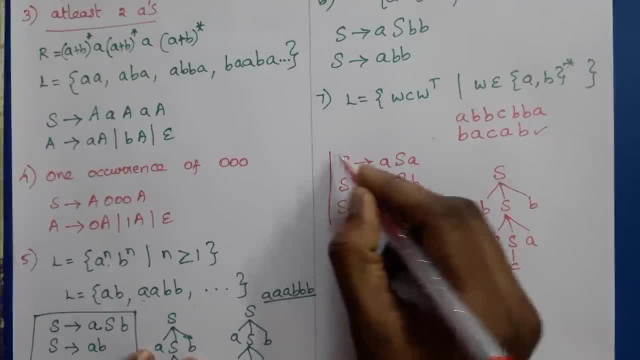 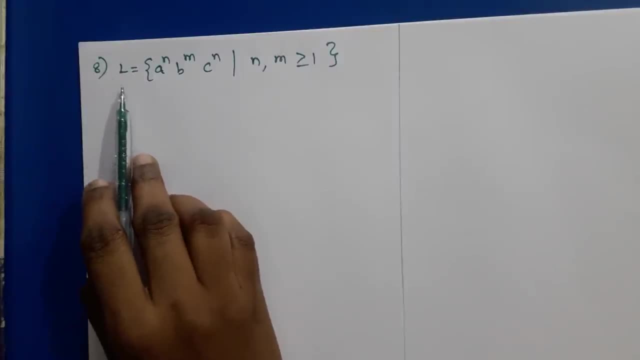 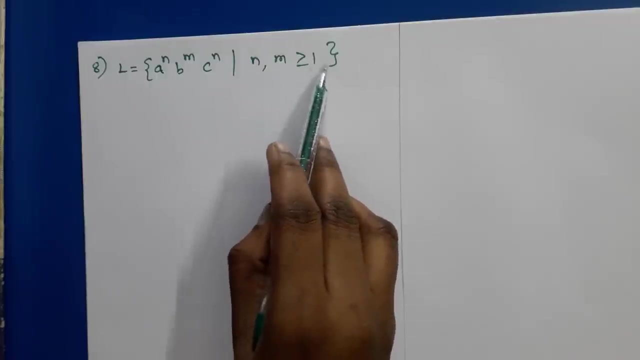 any odd length palindrome. this is the grammar for this particular problem. then next problem is construct cfg for this language. l is equal to a to the power n, b to the power m, c to the power n, such that n and m are greater than or equal to 1. so here number of a's and c's. 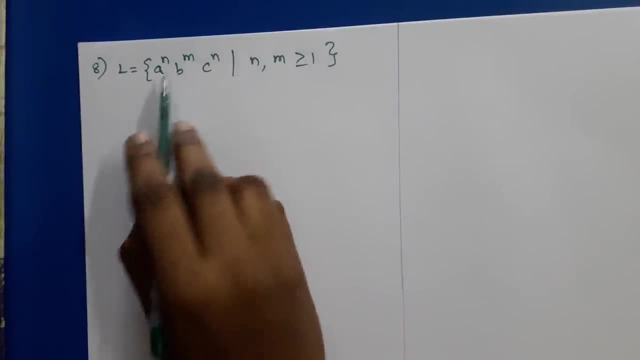 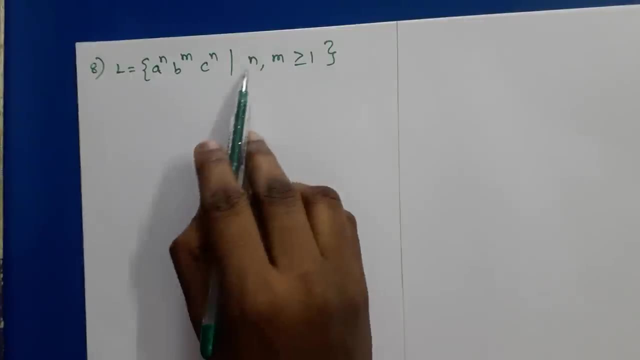 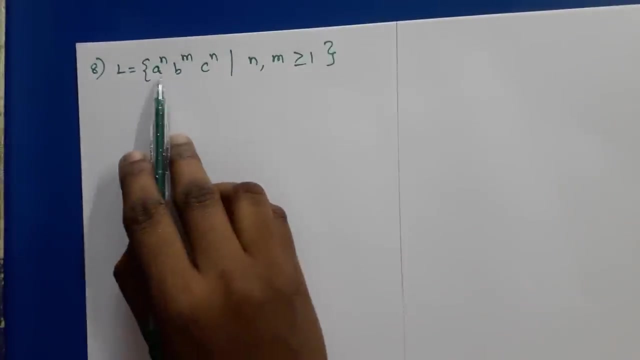 are equal and in between we can have any number of b's, at least one b, okay. so here the number of a, n's and m are greater than or equal to 1. so at least 1 a, followed by 1 b, followed by 1 c, but in all the 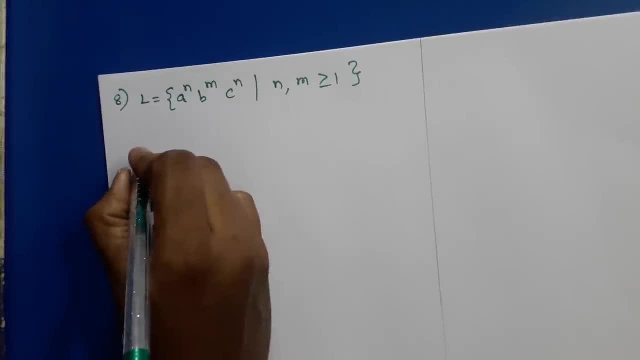 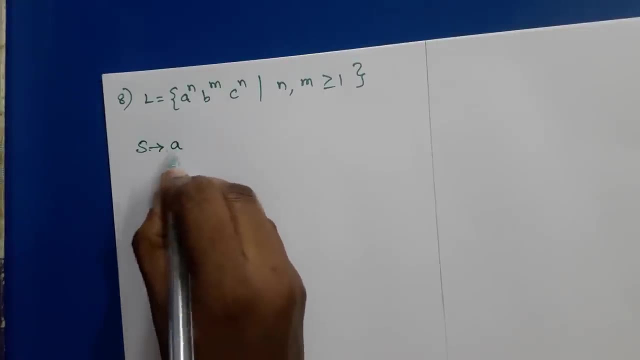 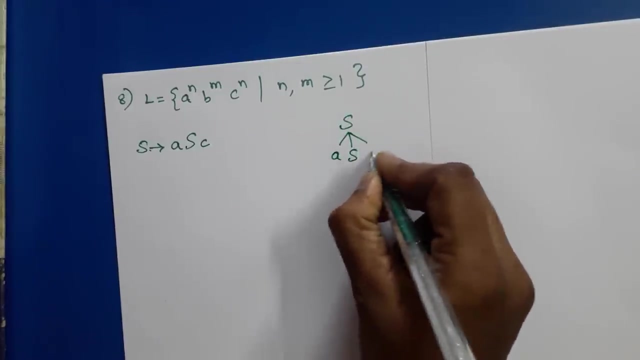 strings. number of a's and c's must be equal, so yes tends to. for 1 a we need to get 1 c right, so a, yes, c. so if we try to construct a parse tree, yes can be replaced by a s, c, a s c, so any number of times. 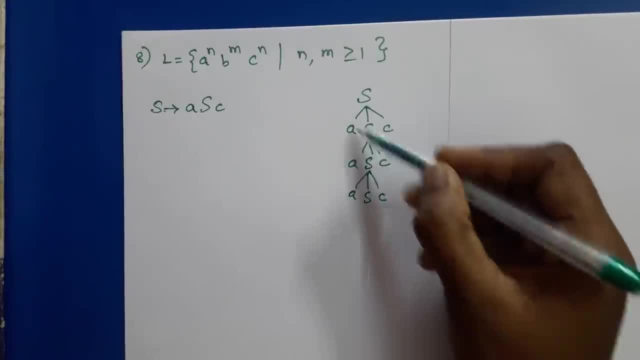 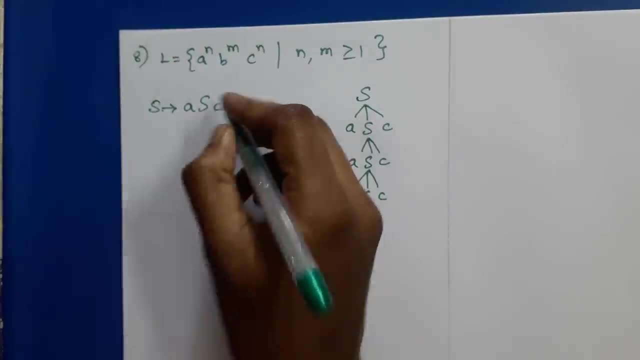 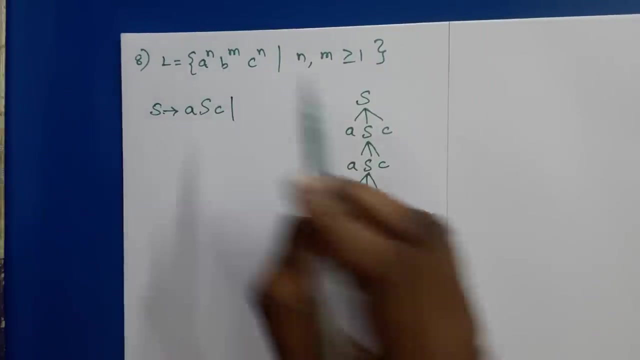 we can apply this, so in this we can get equal number of a's and c's, but in the middle we have to get number of b's right, and so that we have to introduce a new non-terminal symbol for getting the number of b's. and one more thing here: 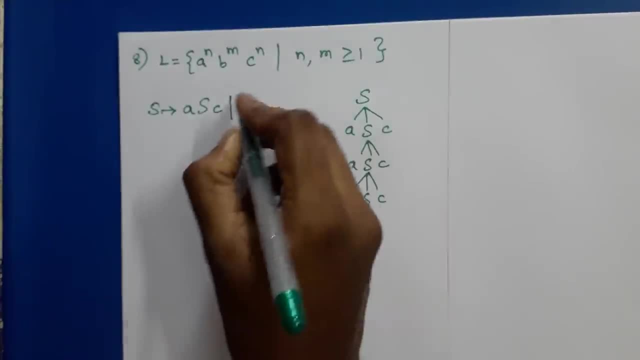 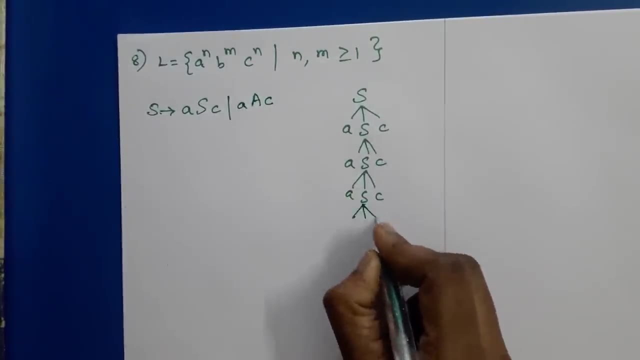 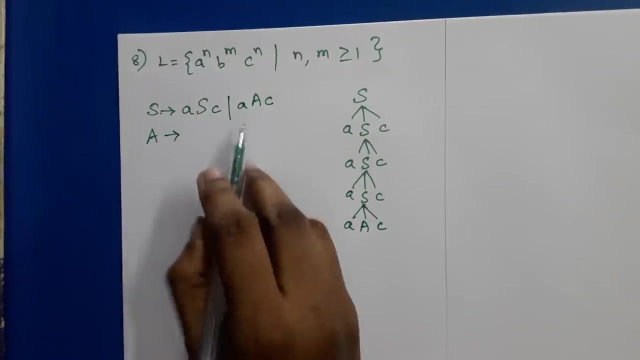 a and c. the number should be at least one, so that we have to write a a c, a a c. so finally we need to replace this by a a c. then only we can apply b here now. now in the middle we need to get a number. 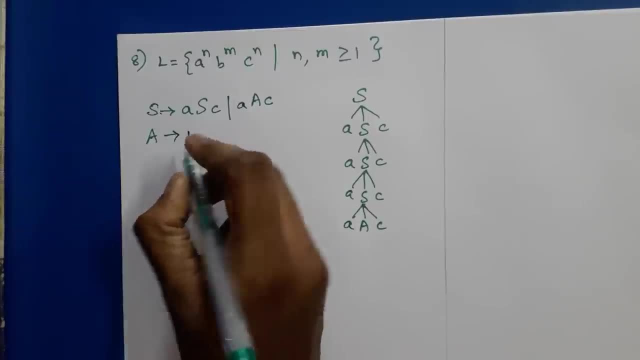 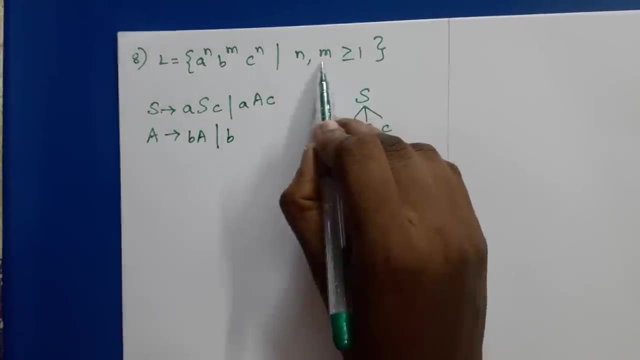 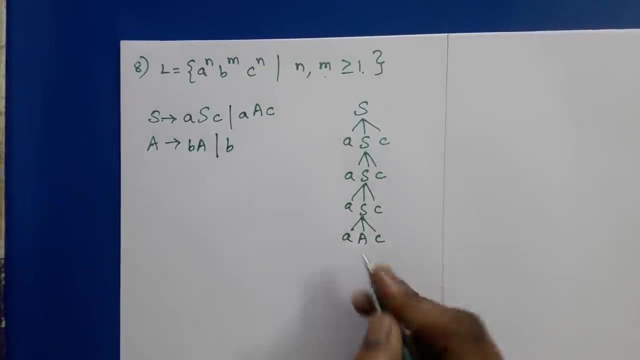 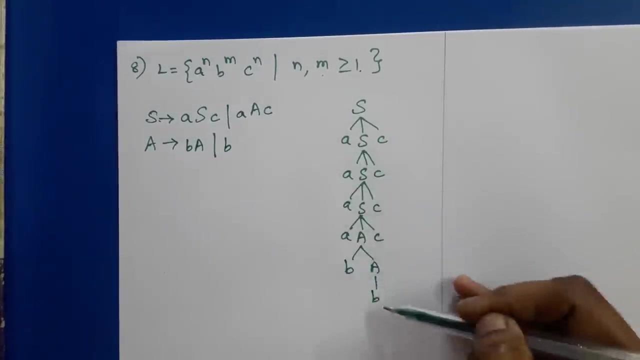 of b's, right. so any number of b's means the production is b, followed by a and b. okay, so here also m is also greater than or equal to 1. so b, a, b, any number of b, a suppose if we want to get 2 b's, here means b, a and b. so in this grammar we have got 4 a's, 2 b's, in this example 4 a's, 2 b. 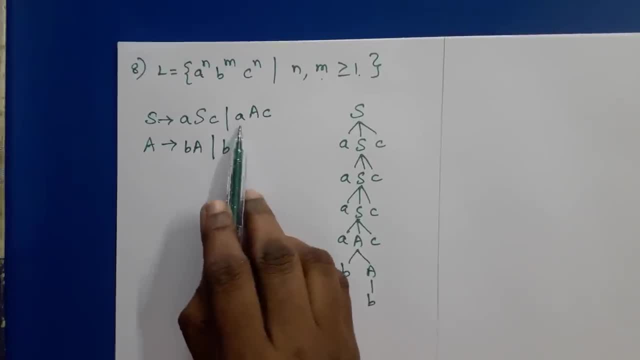 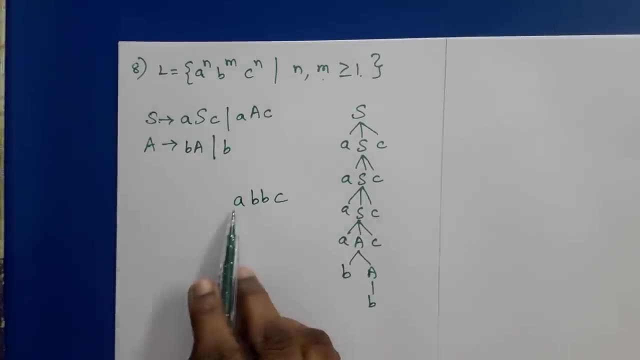 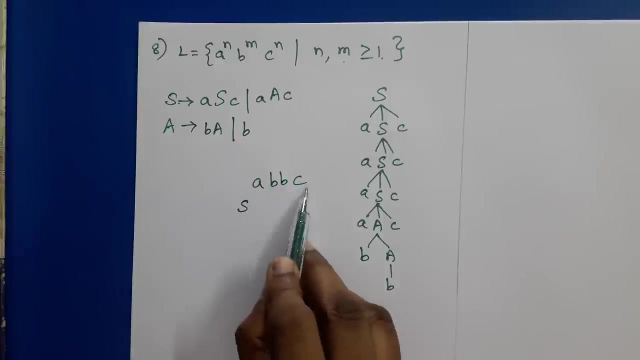 4, c's, similarly we can get. so here, suppose: if we want to get 1 a, 2 b, 1 c, n is 1, m is 2, Then how to construct a parsery S tends to we need only one, A and C. 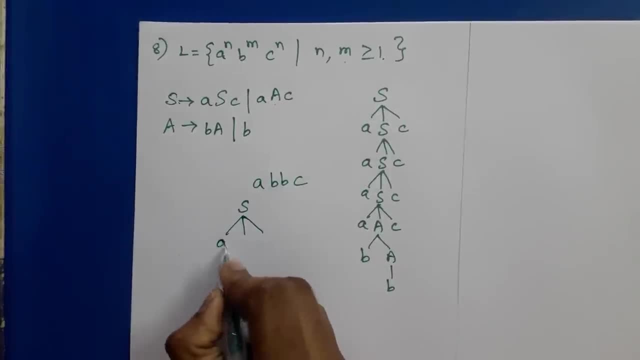 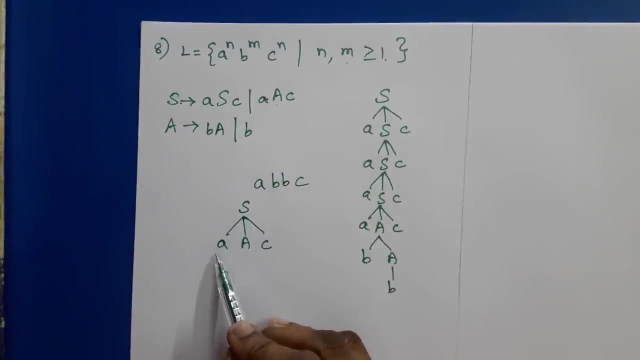 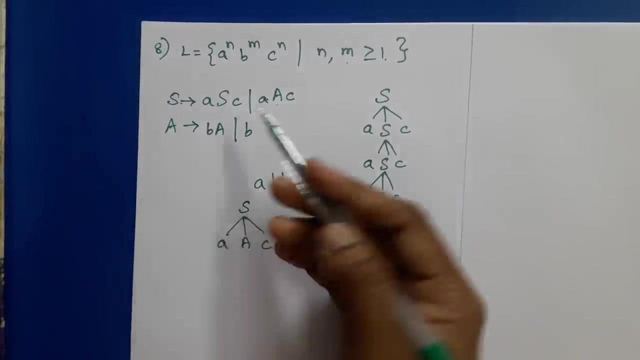 So that we have to use this production directly: A A C. So if we don't write A and C here, then we will write directly: S can be replaced by A and A can be replaced by number of Bs. So we cannot get A and C right. 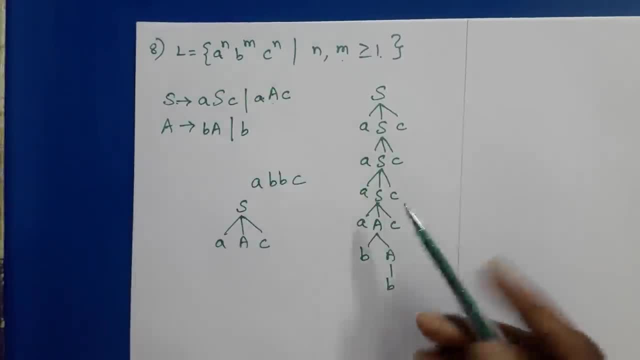 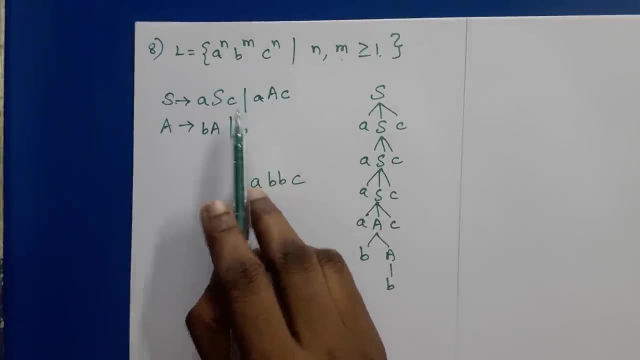 If we don't write A, C here, Simply if we write A, if we replace S by A, then we can get number of Bs alone in this string, So that this A should be preceded by A and it should be followed by C. 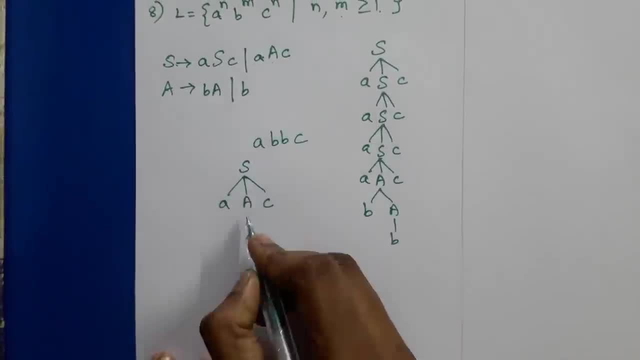 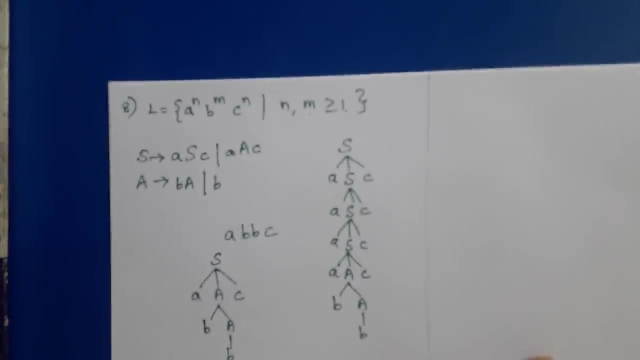 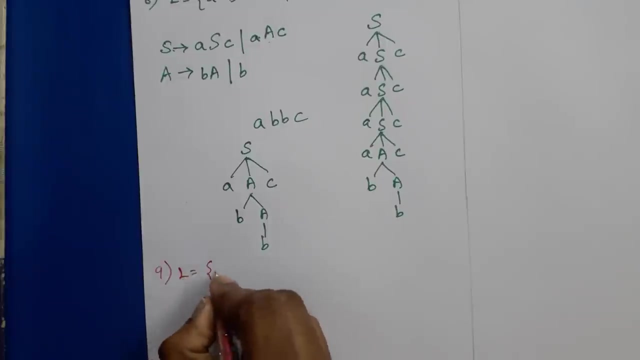 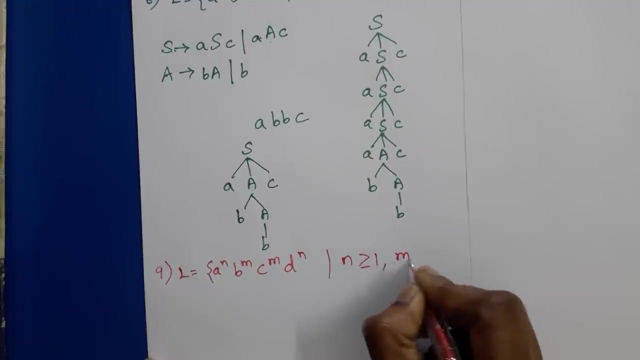 So now S is replaced by A, A, C and two Bs we need. So A must be replaced by B A once, Then this A should be replaced by B. Okay, Similarly We can construct CFG for this grammar, Such that N is greater than or equal to 1 and M is greater than or equal to 1.. 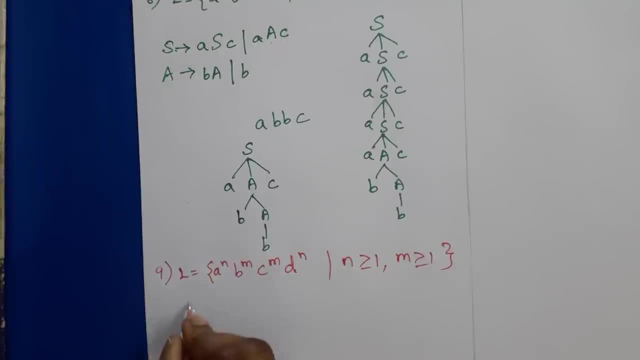 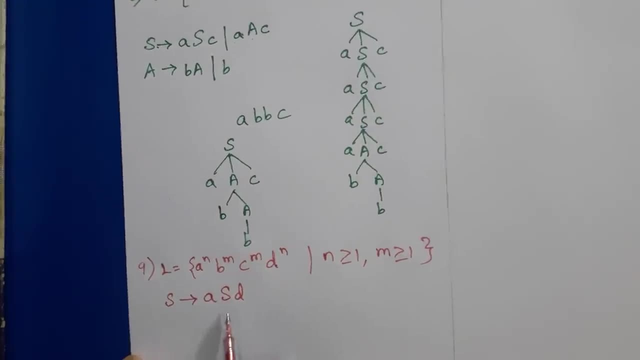 Number of As and Ds must be equal, and Bs and Cs must be equal. So S tends to A, S, D, A and D must be equal. So any number of times we can apply this. But to stop this we have to introduce another non-terminal symbol. 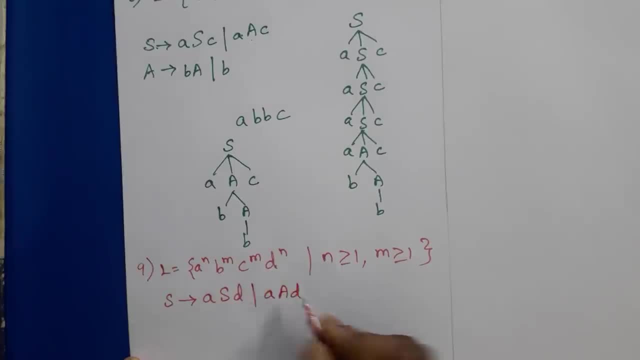 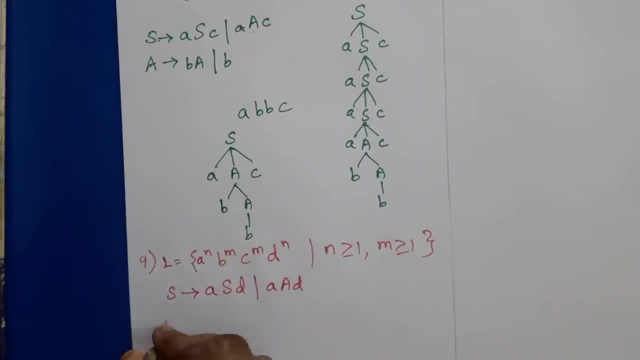 So A, A, D, Right A, S, D should be repeatedly applied. At the end we need to apply this, So this A must be replaced by for A. this A is used for retrieving equal number of Bs and Cs. 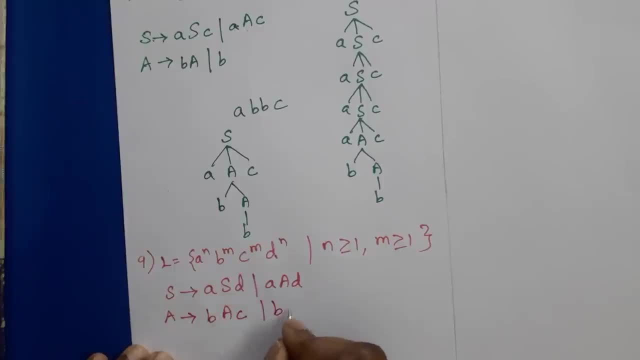 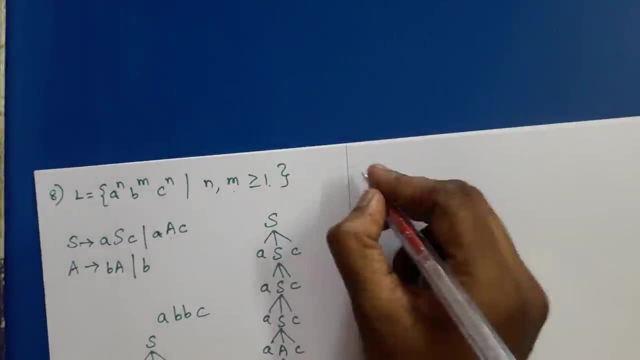 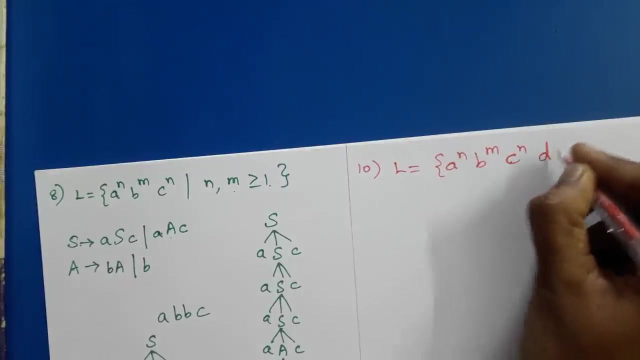 So B A C, bar B C. Okay, So you can take a string and try to draw the parse tree for this grammar. The next one is suppose: A to the power N, B to the power M, C to the power N, D to the power M. 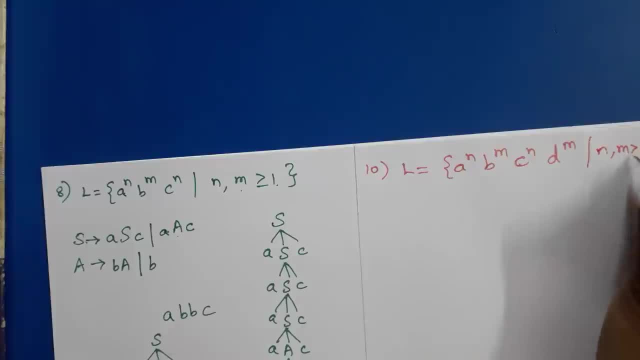 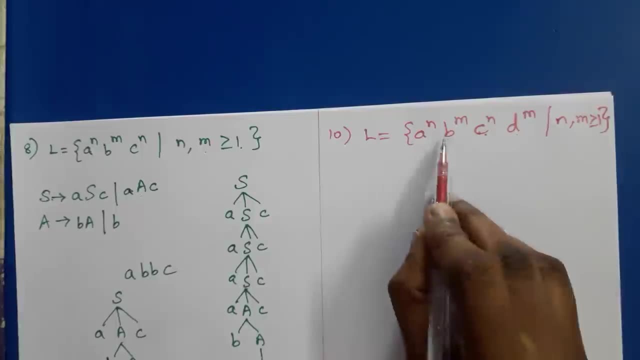 Means: we cannot construct parse tree, for, sorry, We cannot construct CFG for this particular grammar, Because here As and Cs must be equal and Bs and Ds are equal. For this we cannot construct the parse tree. If we try to construct, we will get A, S, C. 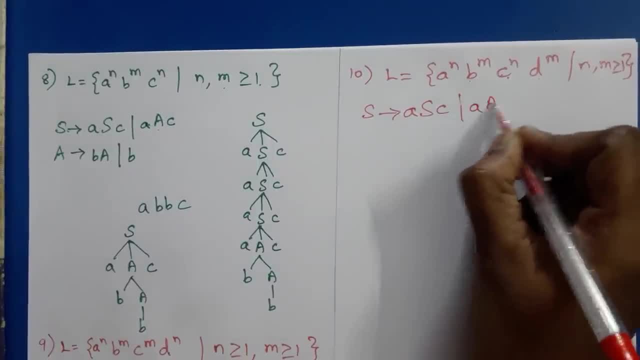 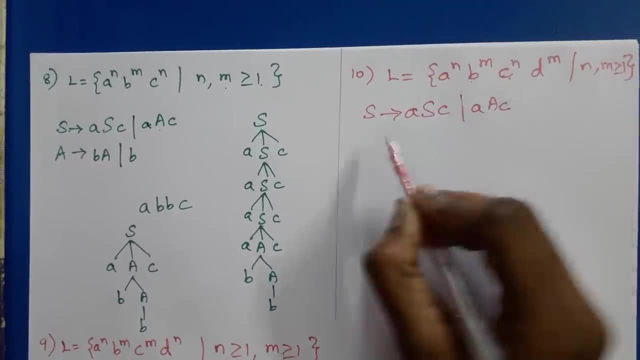 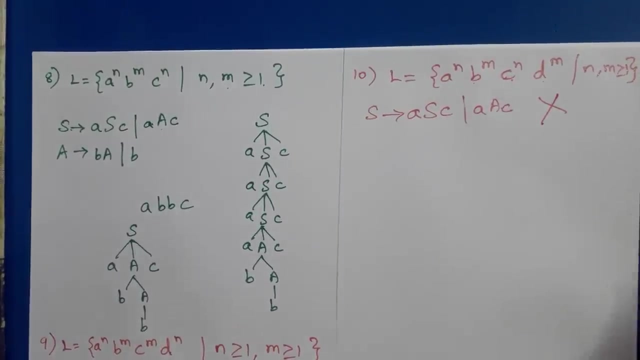 Repeatedly. we need to get this And A, A, C, Then this A. for this A, we have to get B, and Ds must be equal So that we cannot retrieve it, because in between Cs are there, So that this is not a context free grammar. 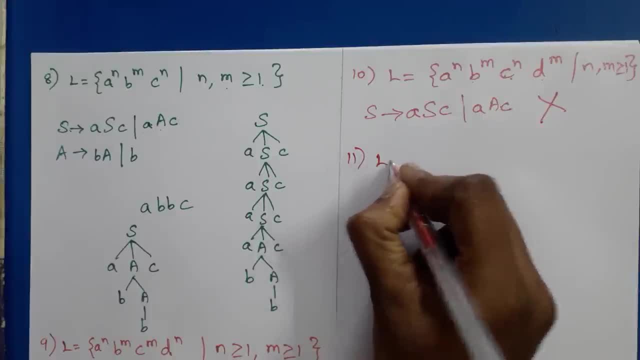 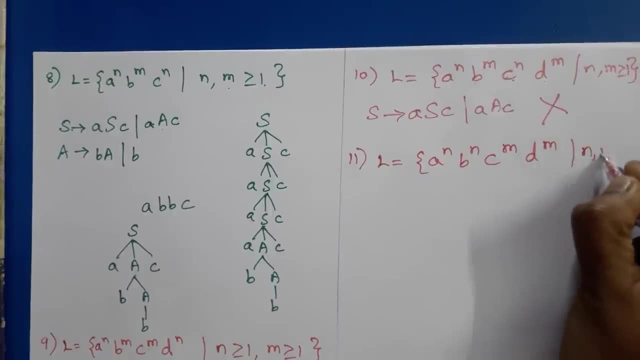 The next one is: L is equal to A to the power N, B to the power N, C to the power M, D to the power M. So for this problem we can construct the parse tree Here. number of As and Bs are equal. 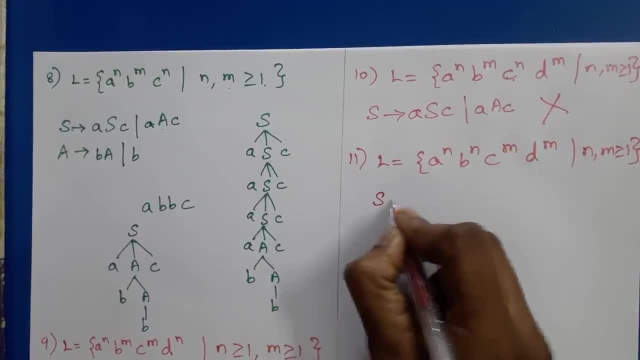 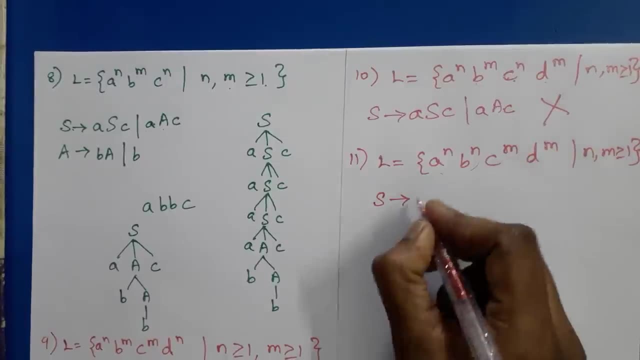 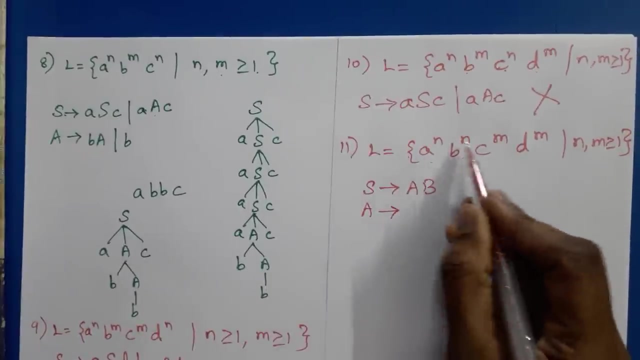 And Cs and Ds are equal. So the thing is we need one variable for getting retrieving this, Another variable for retrieving this, So S can be replaced by two variables: A, B, And for A we need to get number of As and Bs equal right. 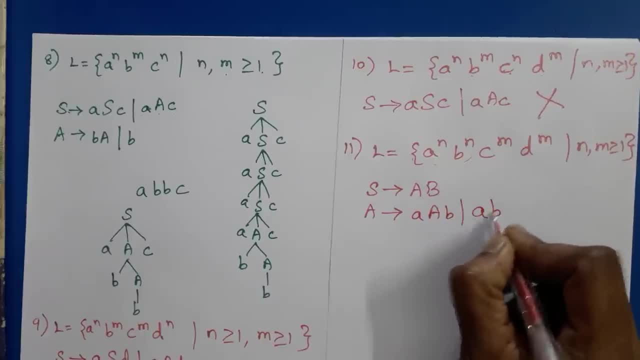 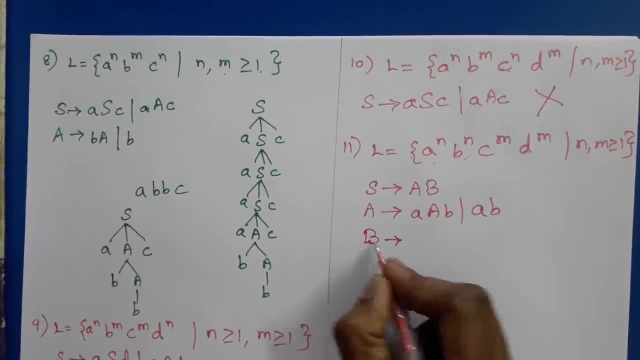 So A A B bar A B, A A B should be repeatedly applied. Finally, it should be replaced by A B. Similarly, B A B should be replaced by C B D bar C- D. okay. 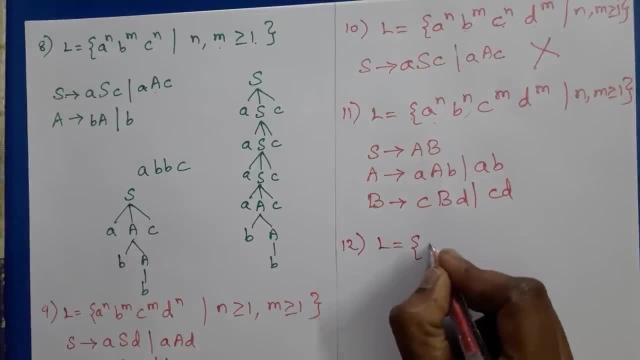 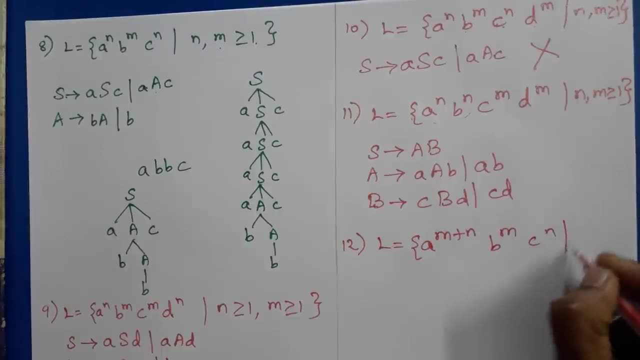 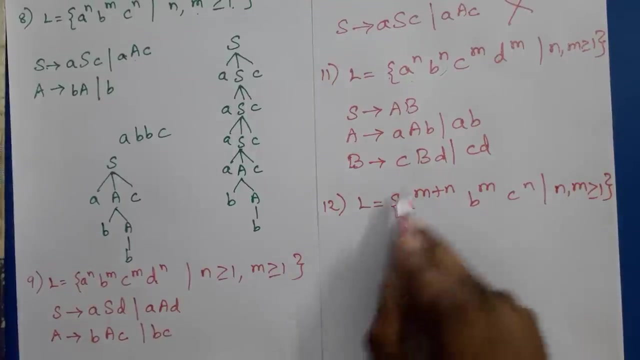 One more: L is equal to A to the power M, plus N, B to the power M, C to the power N. okay, N, comma, M greater than or equal to 1.. So here, first we rewrite this grammar: okay.